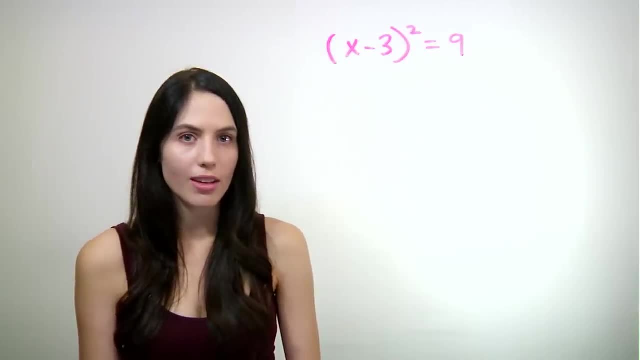 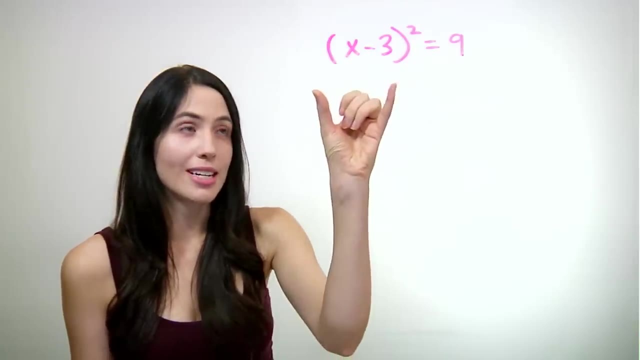 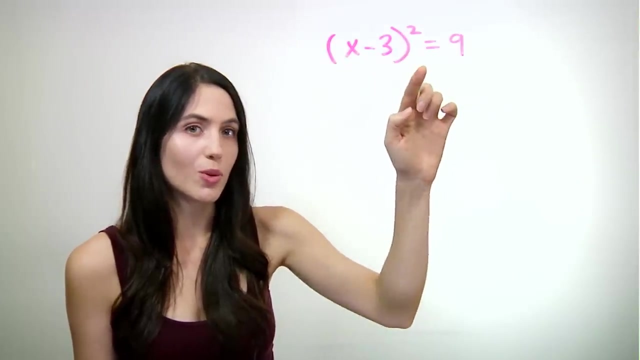 Hi guys, I'm Nancy and I'm going to show you how to solve by completing the square. What is completing the square? It means getting your equation into a neat, perfect square form like this, where you have x plus or minus. a number squared equals another number. Why? 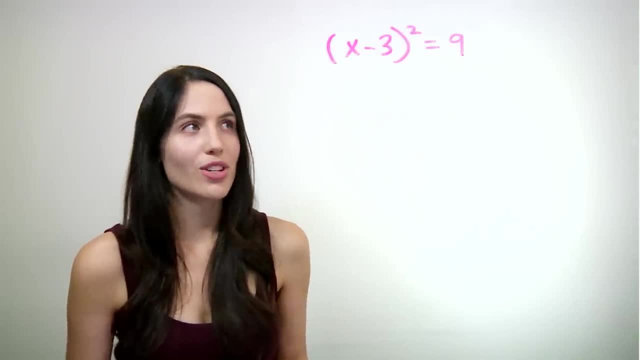 would you want to solve this way? Good question, It's not the best way usually. It's usually easier or faster to solve by factoring, if possible, or quadratic formula, which you can always use, But probably you've been told that you have to solve by completing the square. 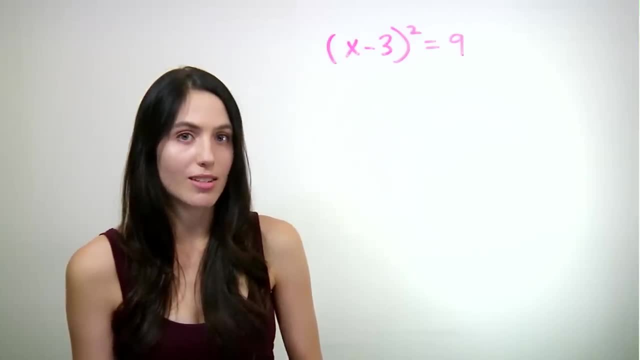 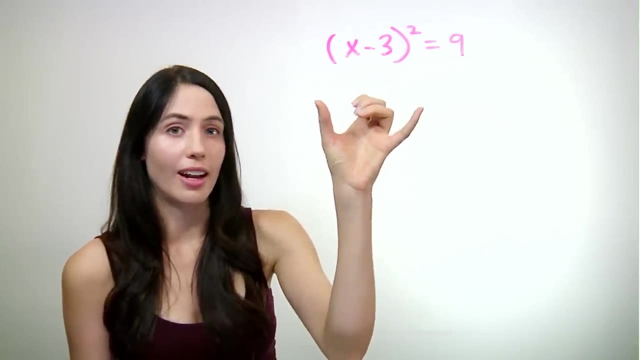 so you need to know how to do it. So I will show you the easiest way to solve by completing the square. Unfortunately, you're not given this form straight away. You have to get it. Usually you're given one of these forms. 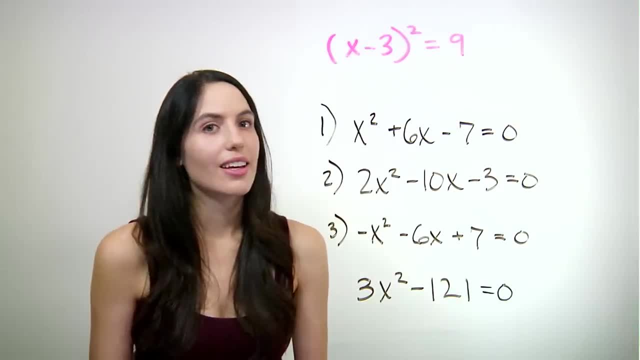 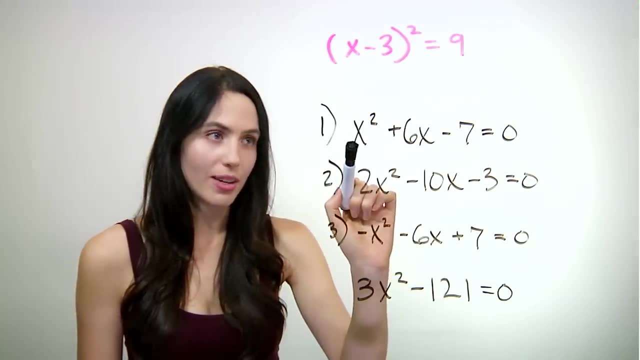 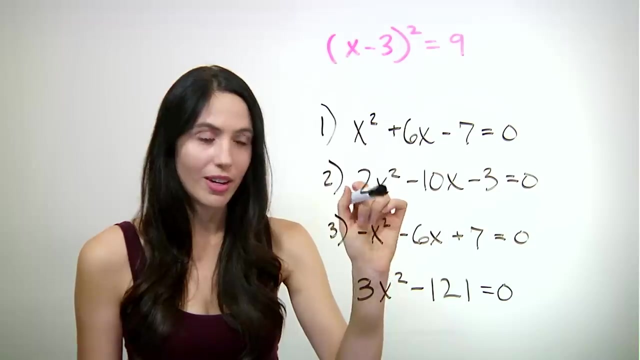 Okay, these are the cases that I'm going to show you. One case is if you have just x squared. positive x squared is your highest term. Another case is if you have a coefficient greater than 1 in front of your x squared, like 2x squared, 3x squared, etc. Third case is if 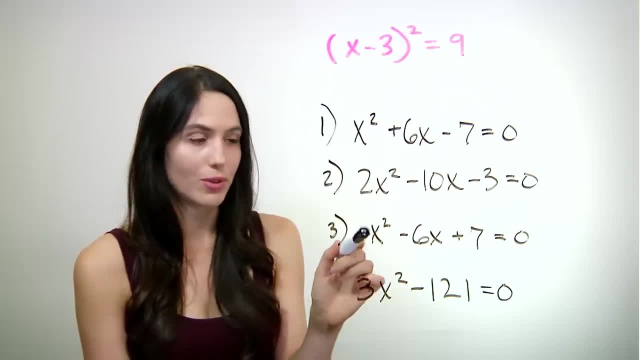 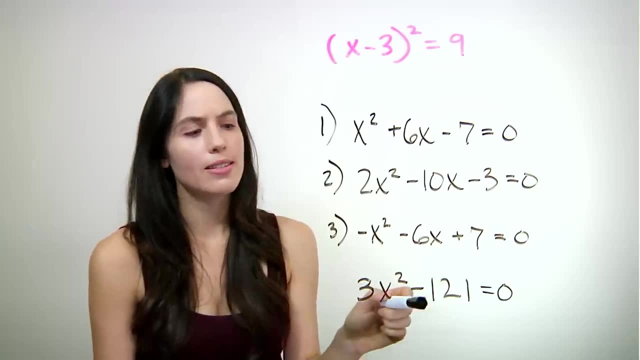 you have a negative coefficient in front of x squared, negative x squared, etc. And this case I put here to show you that you can solve by completing the square. by completing the square, I'm going to show you that if you get something like this that doesn't have an x term, a middle, 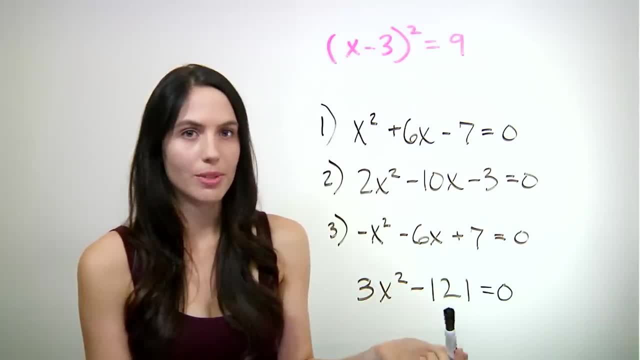 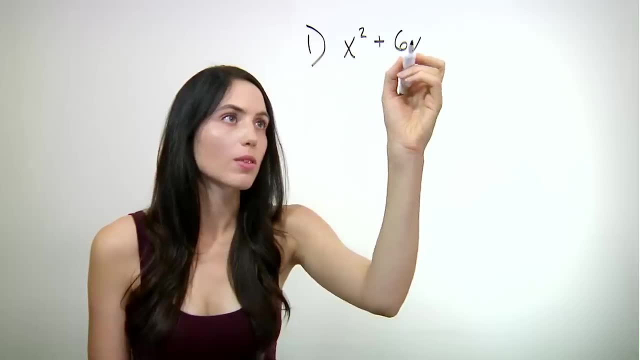 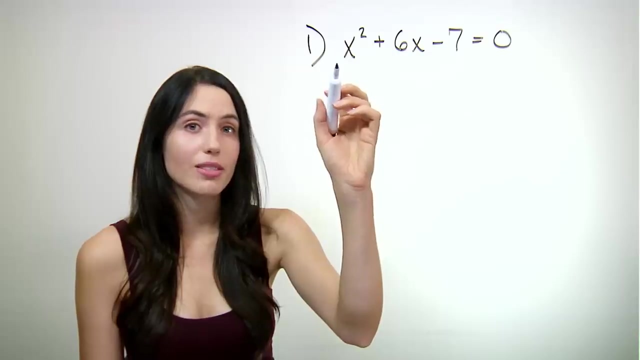 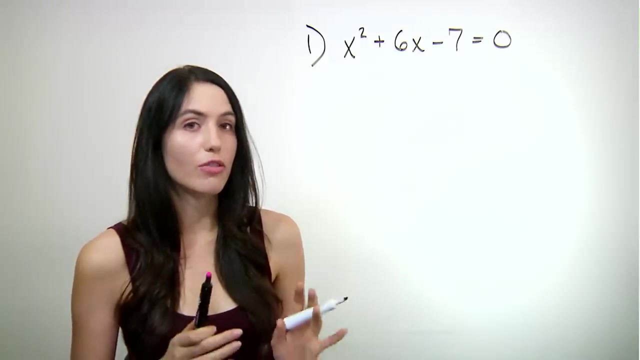 term, you can't complete the square. Sometimes people get confused about that, So really I'm going to show you these three cases. Okay, say you have an equation like this that starts with x squared, positive x squared. The first step actually for all of these: completing the square problems. the first: 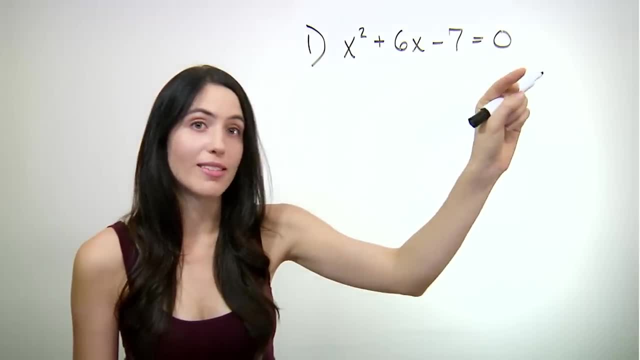 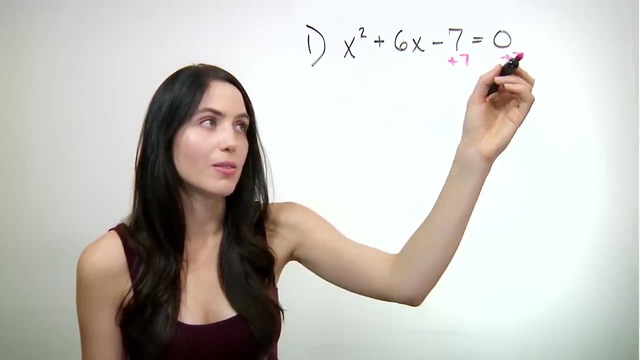 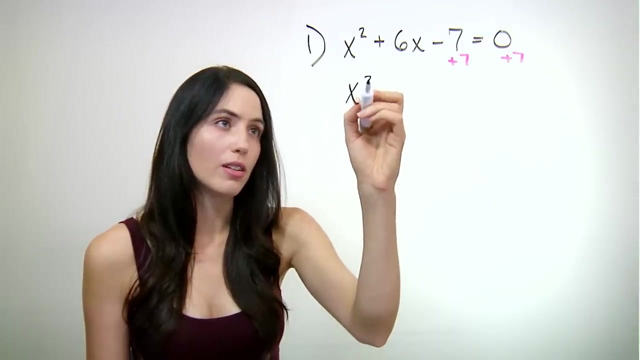 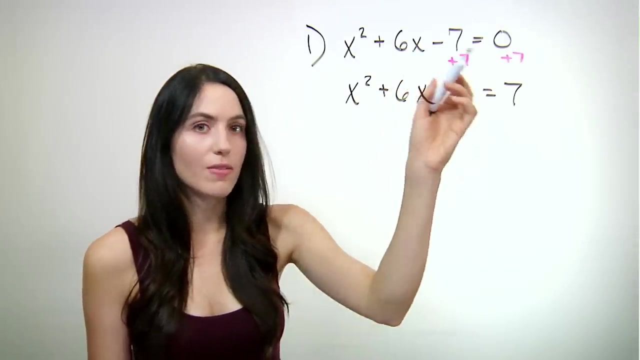 step is to move this constant to the right side. So in this equation the way you would do that is to add 7 to both sides. So always just move that constant over to the right. So what you get is x squared plus 6x equals positive 7.. Notice that the sign flipped. 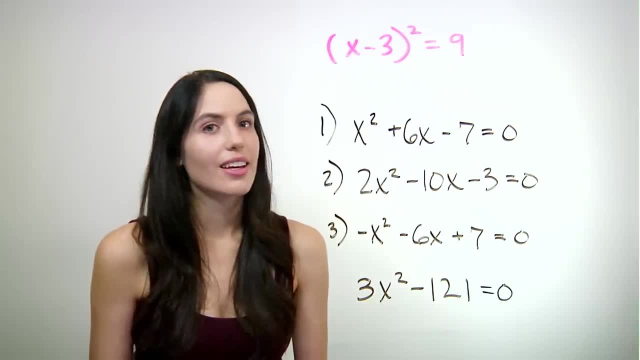 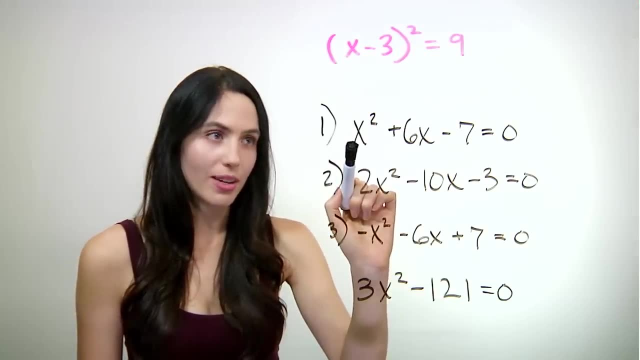 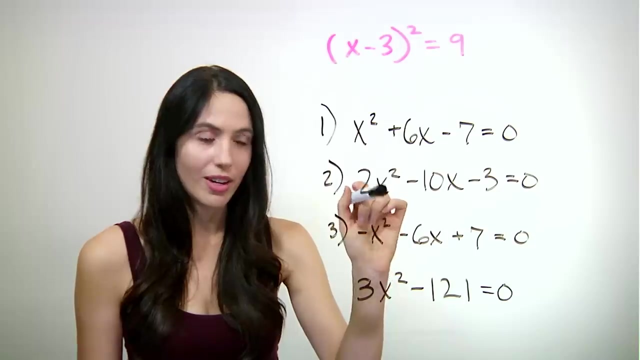 Okay, these are the cases that I'm going to show you. One case is if you have just x squared, positive x squared as your highest term. Another case is if you have a coefficient greater than 1 in front of your x squared, like 2x squared, 3x squared, etc. Third case is if 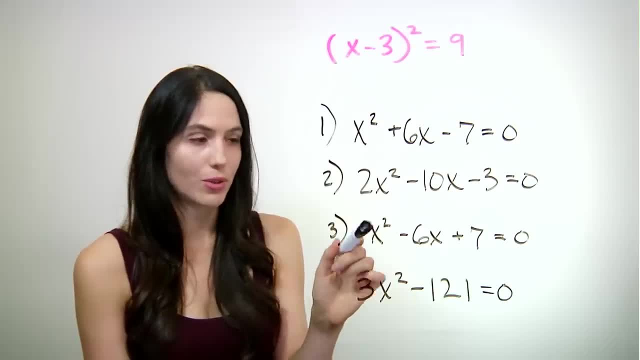 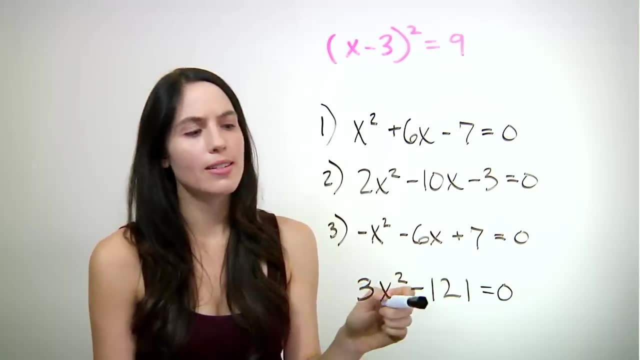 you have a negative coefficient in front of x squared, negative x squared, etc. And this case I put here to show you how to solve by completing the square, by completing the square. So I'm going to show you that if you get something like this that doesn't have an x term, a middle, 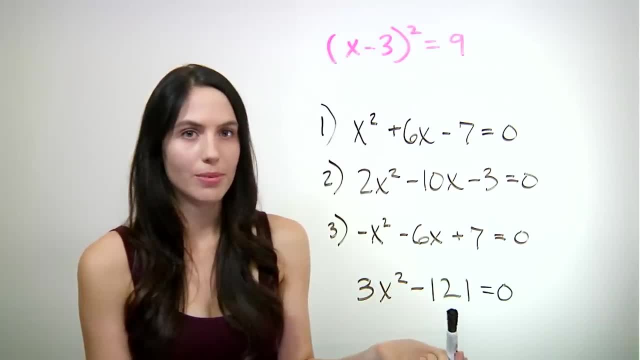 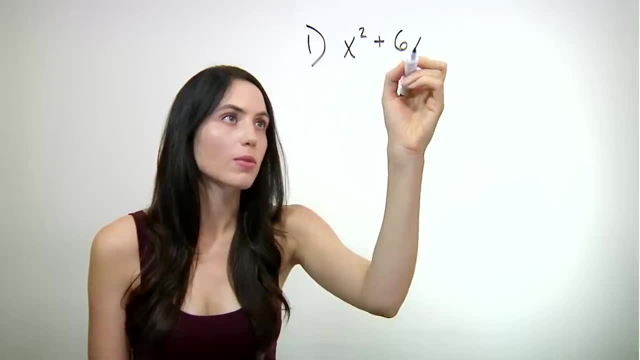 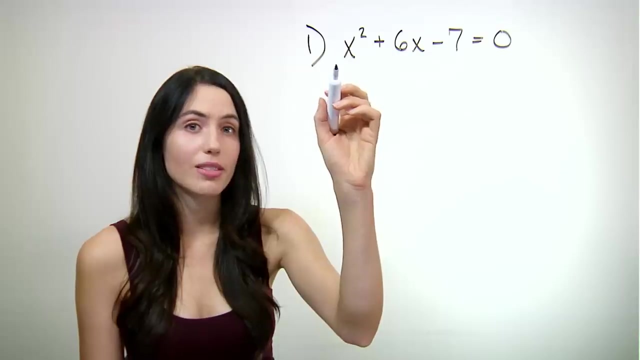 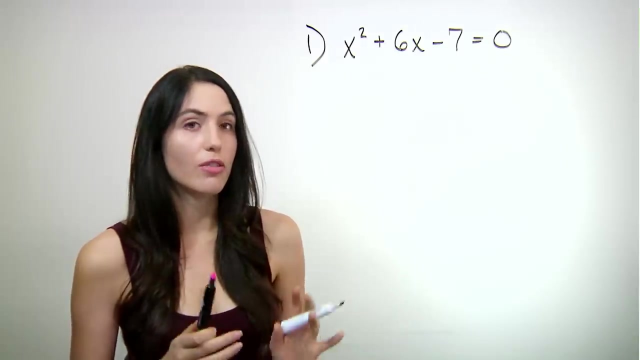 term, you can't complete the square. Sometimes people get confused about that, So really I'm going to show you these three cases. Okay, say you have an equation like this that starts with x squared, positive x squared. The first step actually for all of these: completing the square problems. the first: 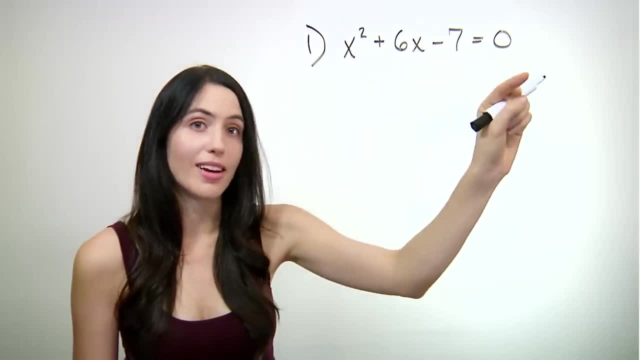 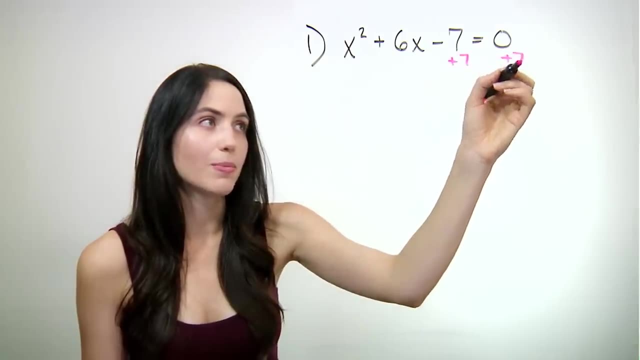 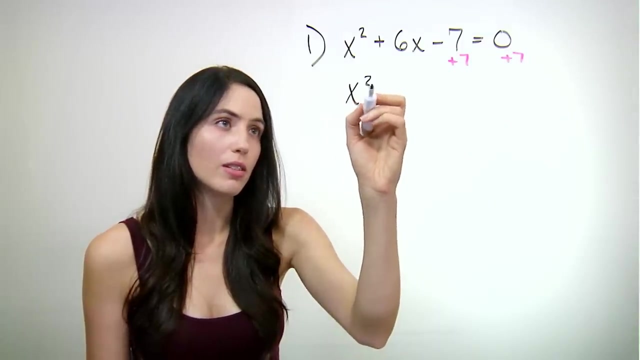 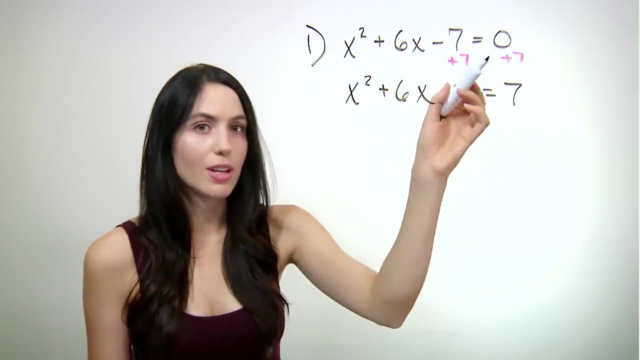 step is to move this constant to the right side. So in this equation the way you would do that is to add 7 to both sides. So always just move that constant over the right. So what you get is x squared plus 6x equals positive 7.. Notice that the sign flipped. That will. 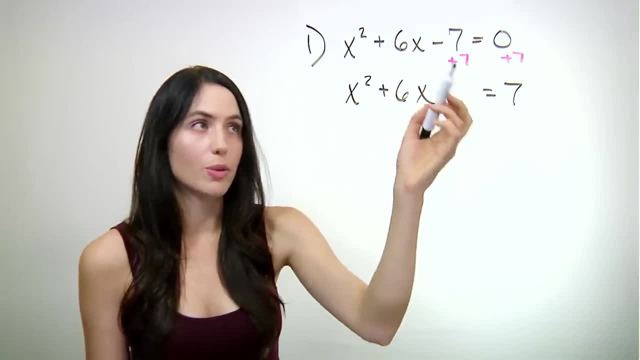 always happen. If it was negative here, it would be positive there. If it was positive here, it would be negative there. If it was positive here, it would be negative there. If it was negative here, it would be negative on the right side. 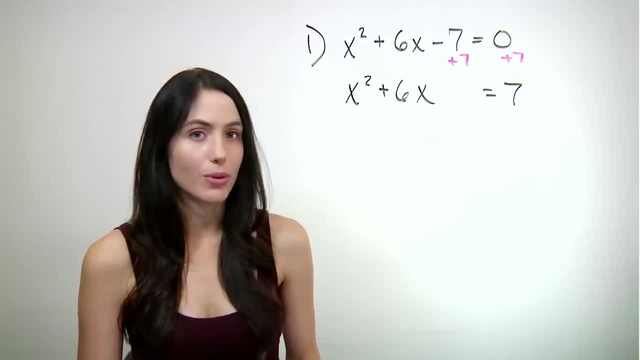 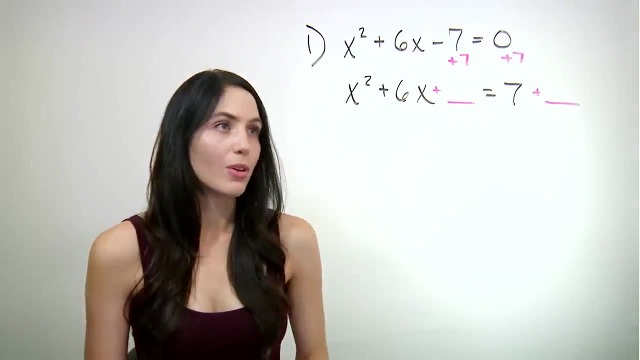 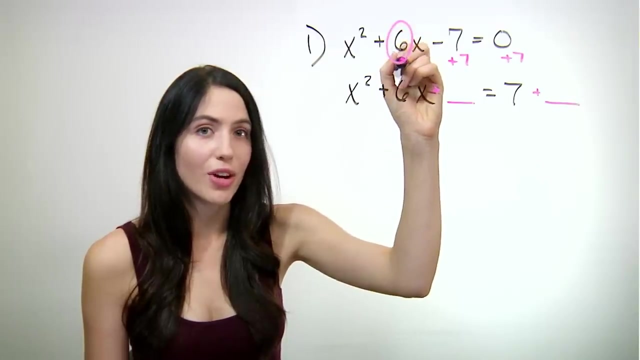 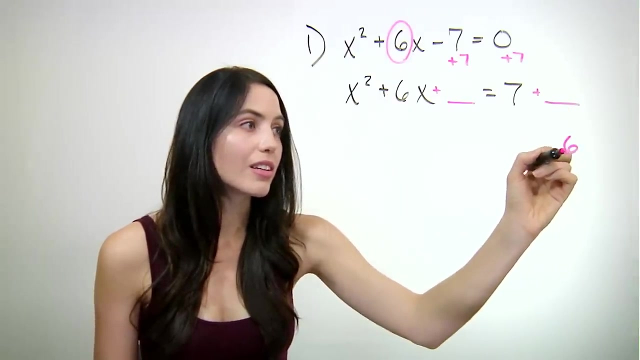 The next step is to add a number to both sides, So you're going to have plus something and plus something. What number do you add? You always get the number by taking the coefficient of x, the coefficient of the middle term, in this case 6, dividing it by 2, and then 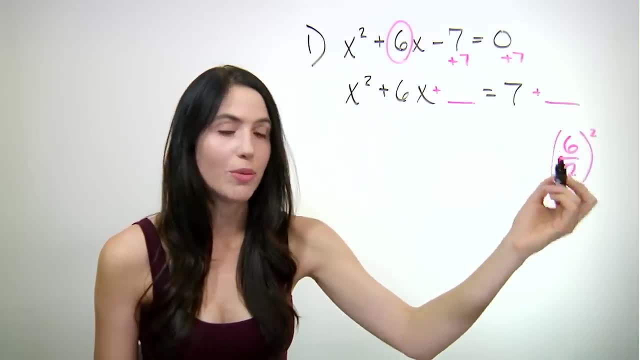 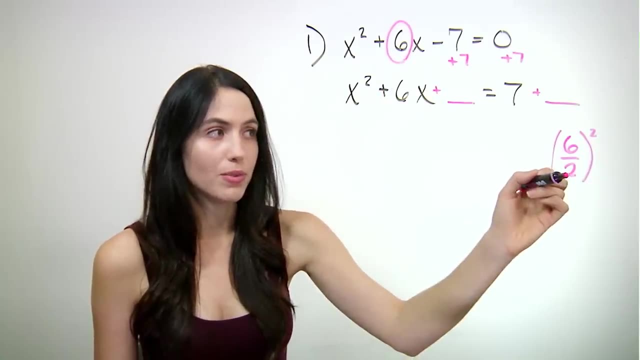 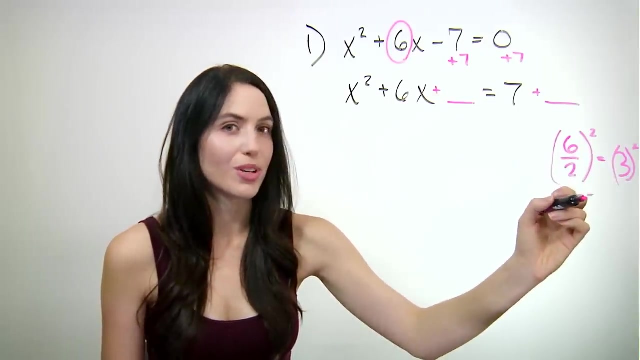 squaring it, And that will be what you'll add to the left and right side. So in this case it's 6 divided by 2 squared, which simplifies to 3 squared, which equals 9.. So we'll be. 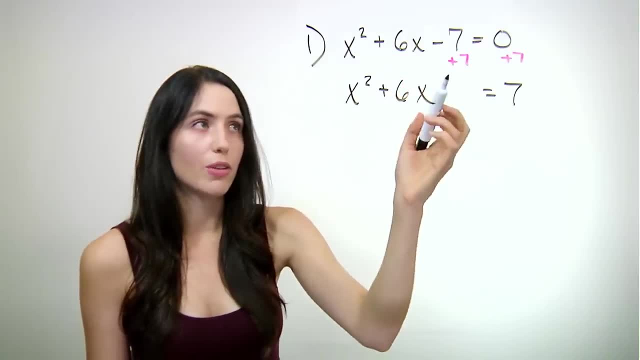 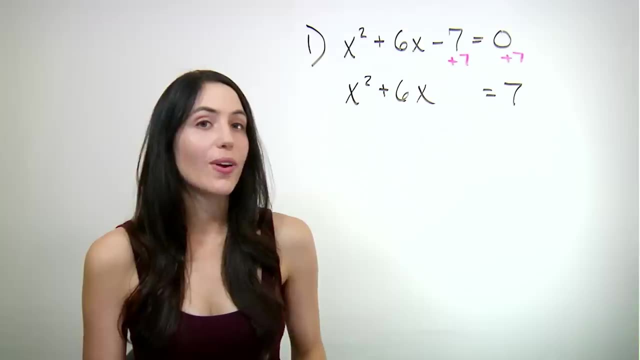 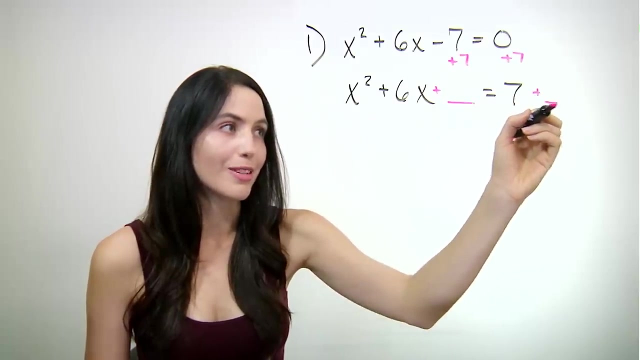 that will always happen. If it was negative here, it will be positive there. If it was This, positive here would be negative on the right side. The next step is to add a number to both sides, So you're going to have plus something and plus something. 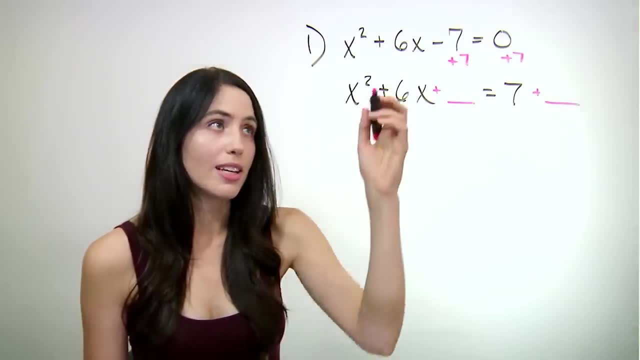 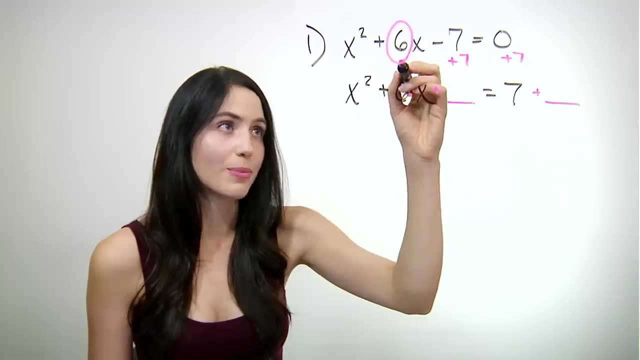 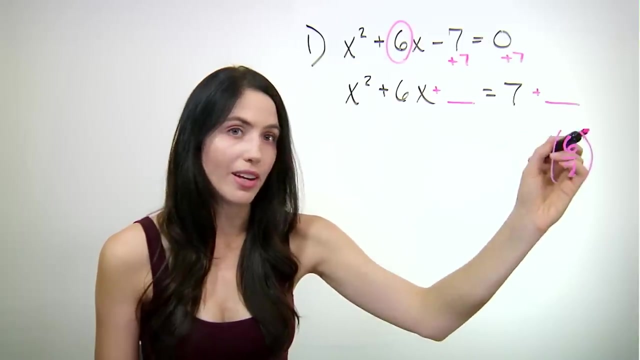 What number do you add? You always get the number by taking the coefficient of x, the coefficient of the middle term, in this case 6,, dividing it by 2, and squaring it, And that will be what you'll add to the left and right side. 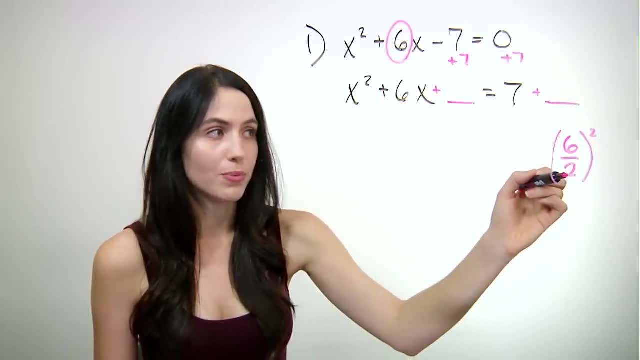 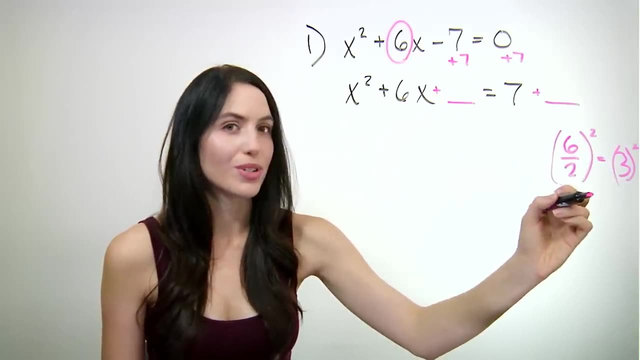 So in this case it's 6 divided by 2, squared, which simplifies, to 3, squared, which equals 9.. So we'll be adding 9 to the left side and the right side. So here we go. 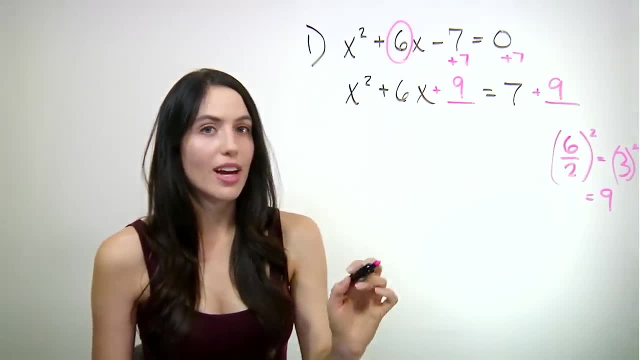 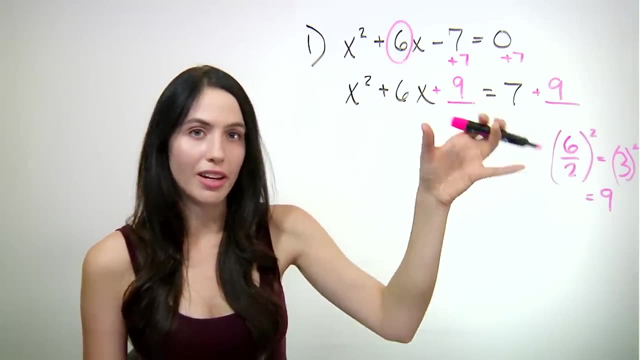 Here we fill in plus 9,, plus 9.. We've added the same thing to both sides. What you do to one side, you must do to the other, so that we don't change the overall value of the equation, so that it's balanced. 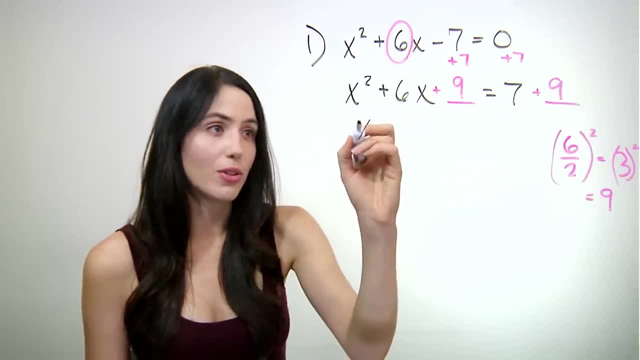 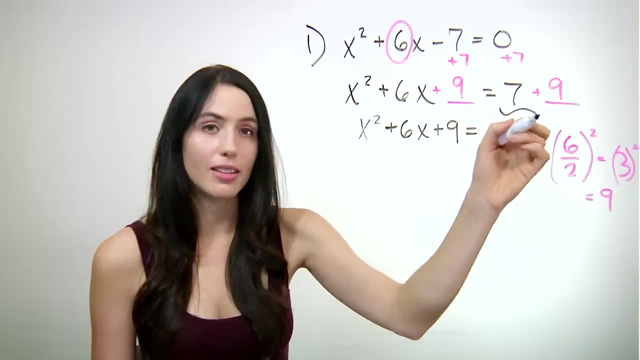 Okay, so then the next line that simplifies to x squared plus 6x plus 9.. And the right side. we can combine these numbers into 16.. 7 plus 9, 16.. Why did we do that? 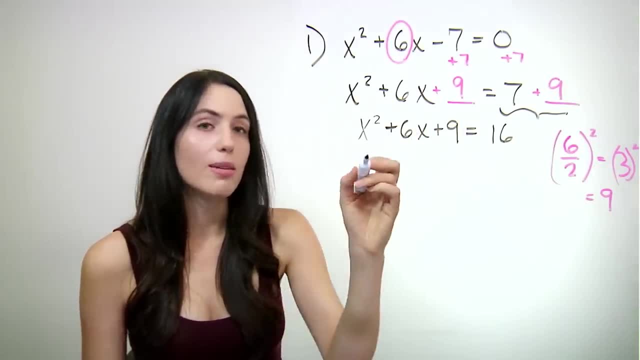 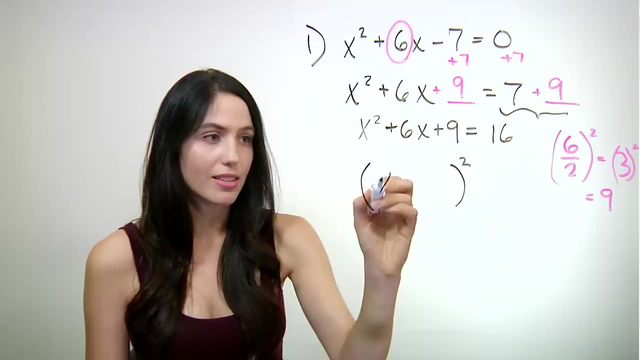 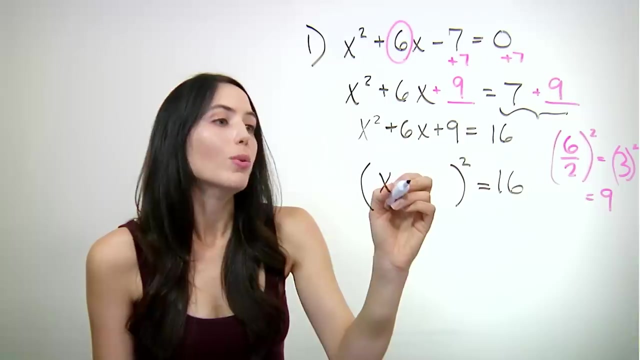 Why did we add another number? Why did we add a number to both sides? The only reason is so that immediately after we can write the left side as a perfect square, x plus or minus. some number squared equals 16. still, The number you write here is always half of what the middle coefficient was. 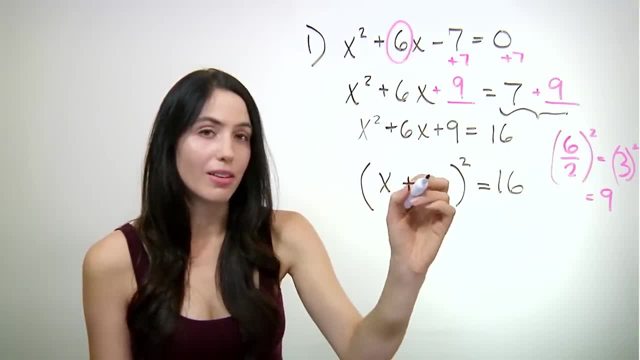 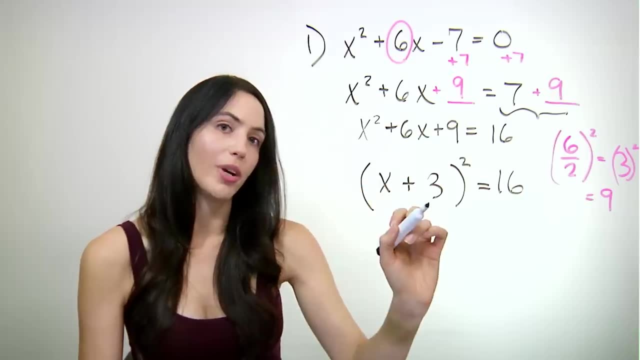 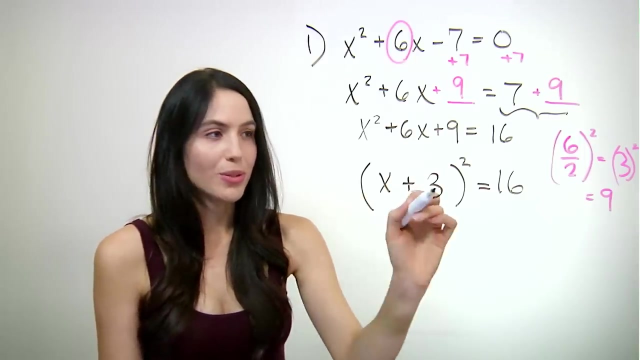 So in this problem it was 6 over 2, positive 3.. If this were negative 6, you would put negative 3.. So always in the perfect square, decide: use half of what the middle coefficient was. So now we have x plus 3, squared equals 16.. 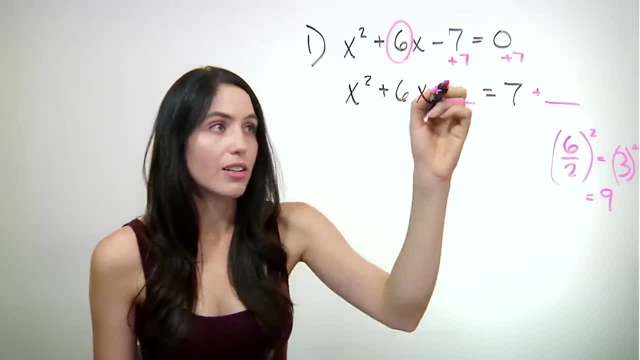 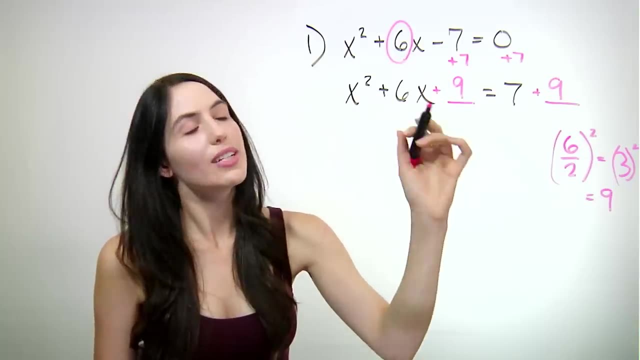 adding 9 to the left side and the right side. So here we fill in plus 9, plus 9.. We've added the same thing to both sides. What you do to one side you must do to the other, so that we don't change the overall. 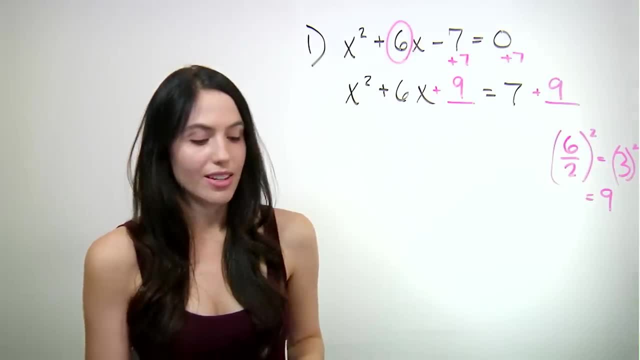 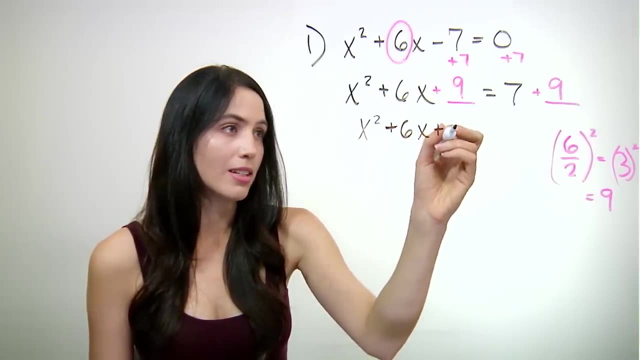 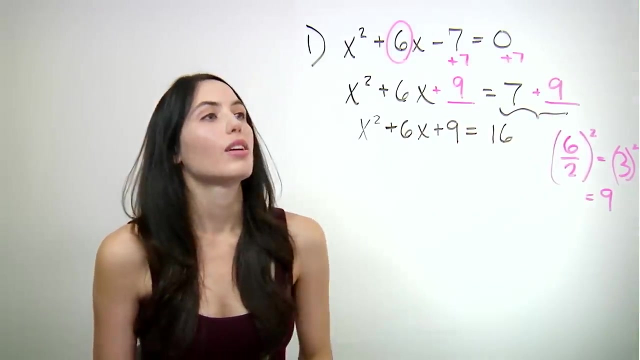 value of the equation so that it's balanced. OK, So in the next line that simplifies to x squared plus 6x plus 9.. And the right side: we can combine these numbers into 16.. 7 plus 9, 16.. Why did we do that? Why did we add? 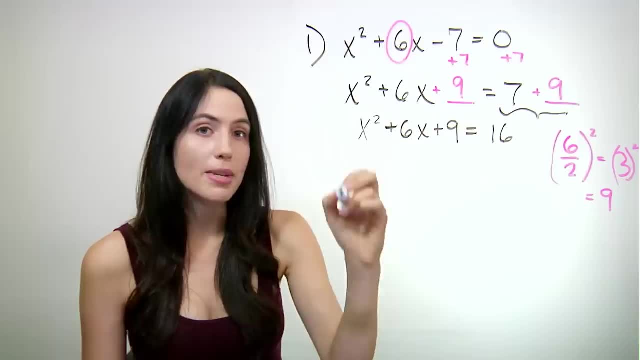 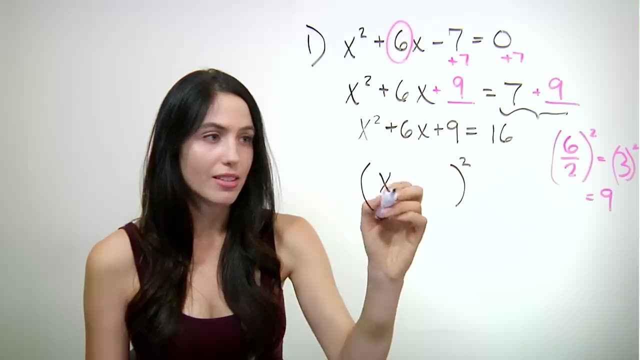 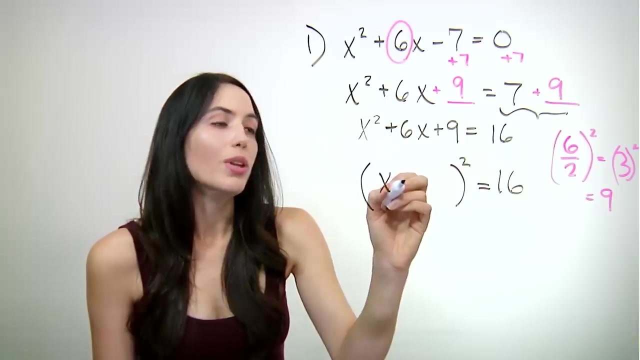 a number to both sides. The only reason is so that immediately after we can write the left side as a perfect square: x plus or minus. some number squared equals 16. still, The number you write here is always half of what the middle coefficient was. So 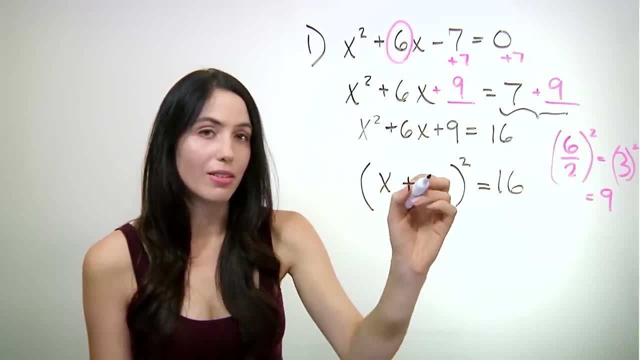 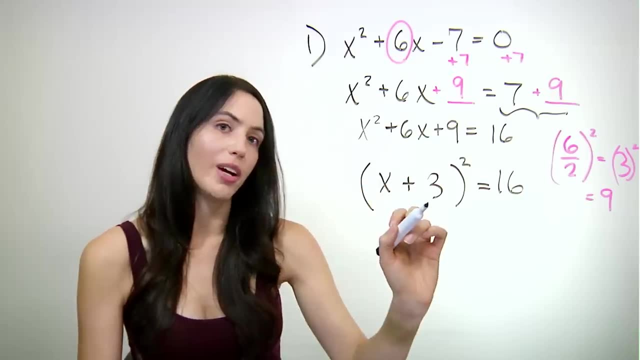 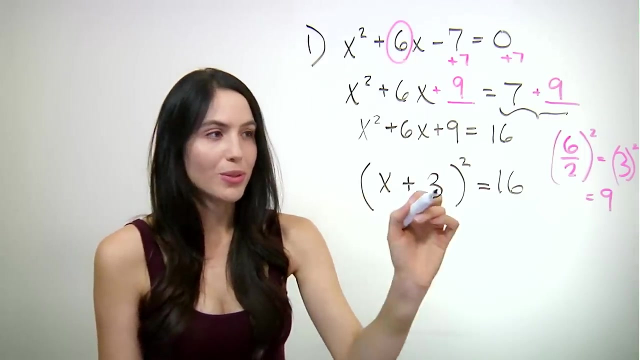 in this problem it was 6 over 2, positive 3.. If this were negative 6, you would put negative 3.. So always in the perfect square, Decide: Use half of what the middle coefficient was. So now we have x plus 3, squared equals 16.. That's great, You've completed the square. 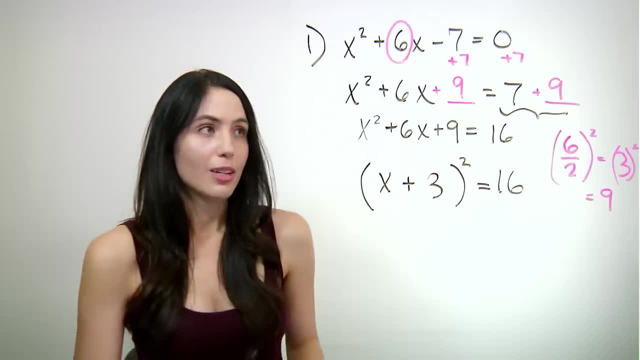 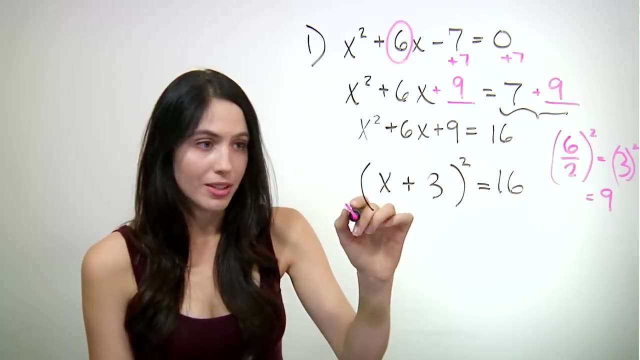 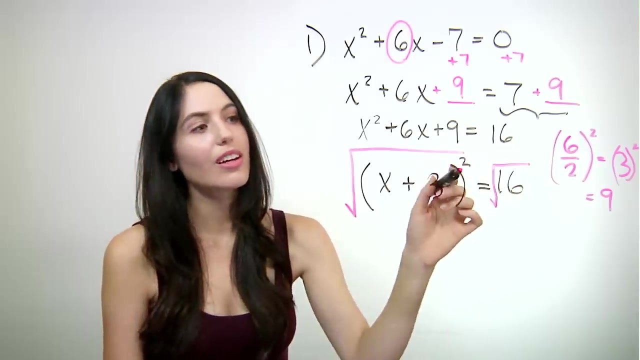 You have something that will be very easy to solve now, And the whole point of doing that was so that you can square root both sides in order to solve. We can literally draw a big square root on the left side and a square root on the right side. Be careful. 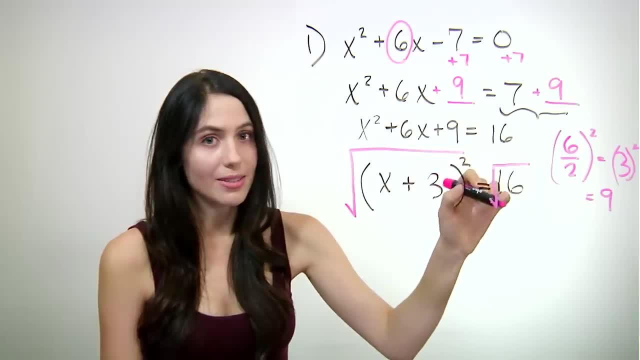 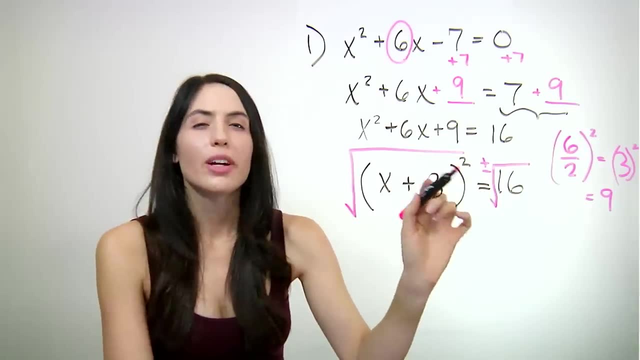 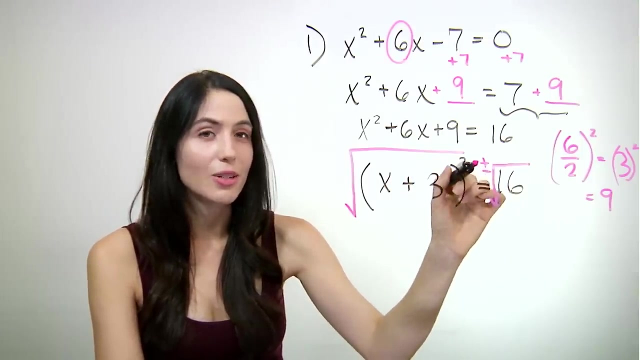 Because when you square root a constant on one side, you actually get two solutions: positive and negative. It's very important And many people forget this, So try to remember. when you square root the side that has the constant, you immediately have two solutions. 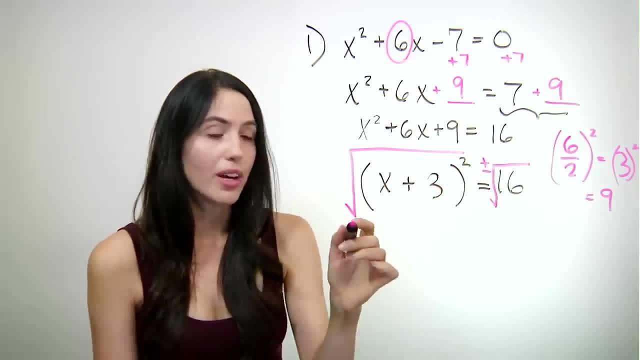 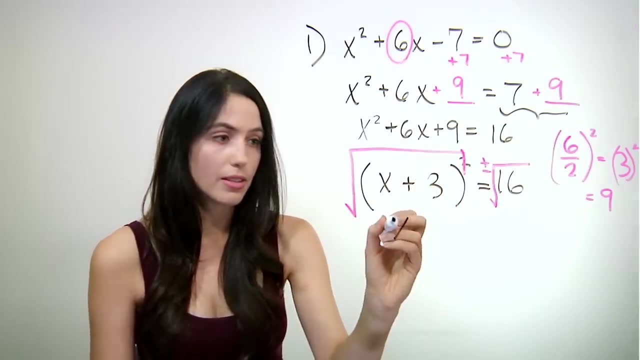 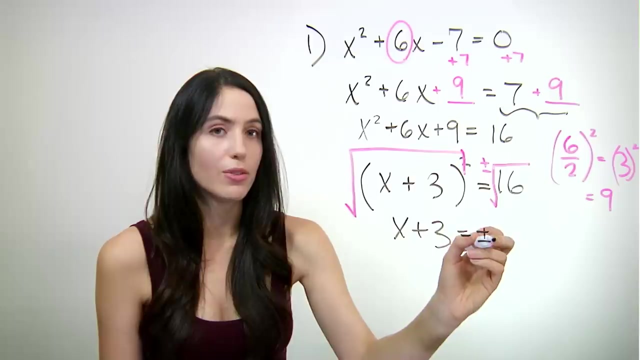 possible the positive and the negative version. Okay, On the left side, meanwhile, what that does is gets rid of the square, So you just have x plus 3. squared equals 16.. So that's going to be x plus 3, what was inside the parentheses equals positive and negative. 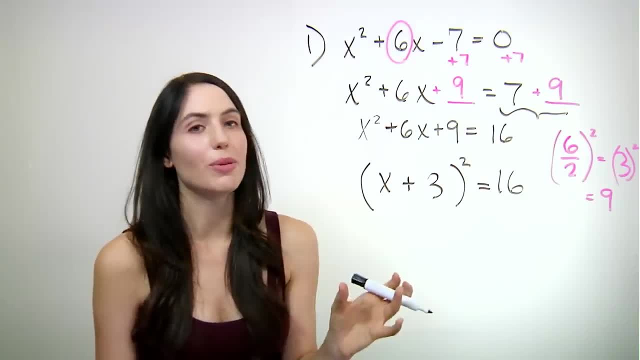 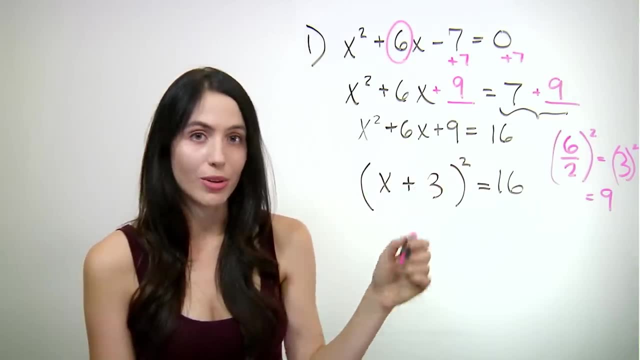 That's great. You've completed the square. You have something that will be very easy to solve now, And the whole point of doing that was so that you can square root both sides in order to solve. We can literally draw a big square root. 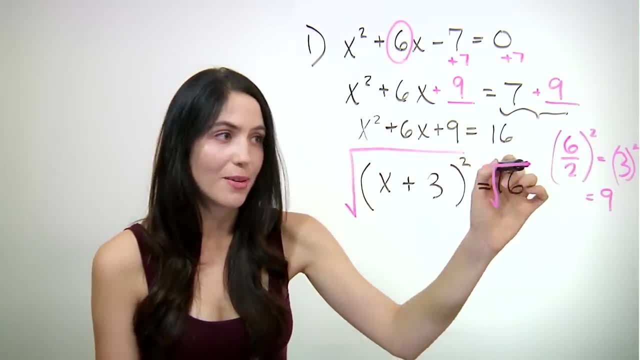 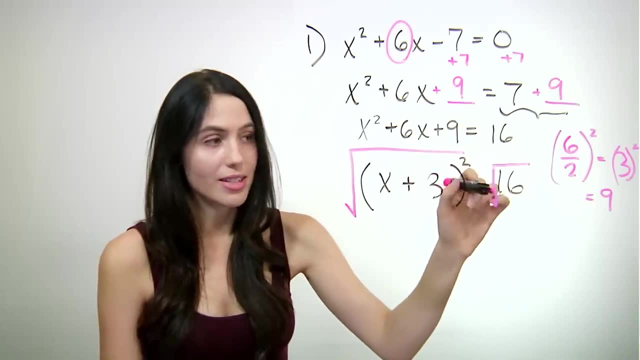 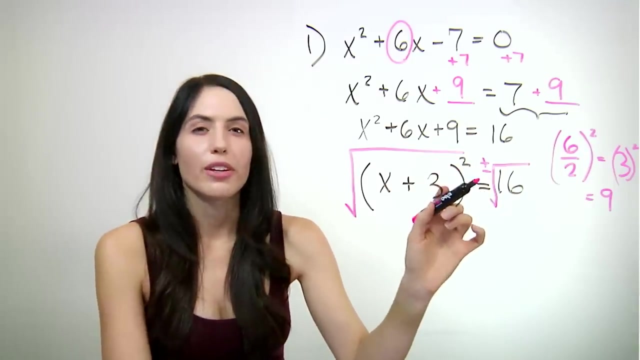 A square root on the left side and a square root on the right side. Be careful, because when you square root a constant on one side, you actually get two solutions: positive and negative. It's very important and many people forget this. 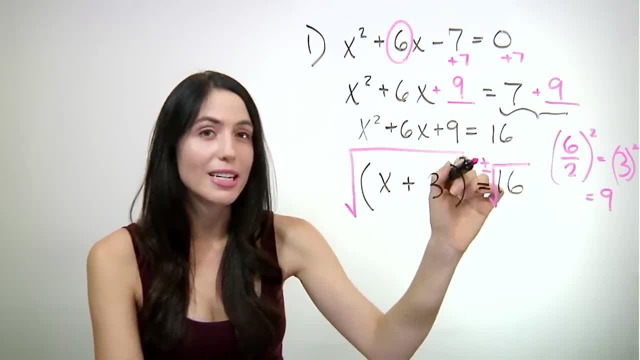 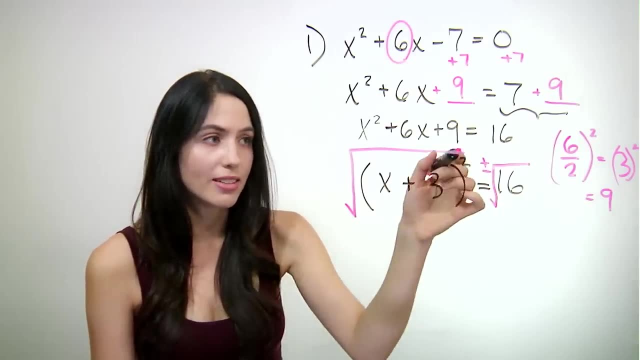 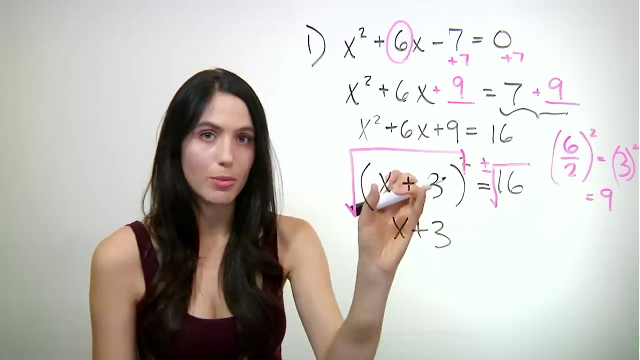 So try to remember: when you square root, the side that has the constant, you immediately have two solutions possible: the positive and the negative version. Okay, On the left side, meanwhile, what that does is gets rid of the square, So you just have x plus 3, what was inside the parentheses equals positive and negative. 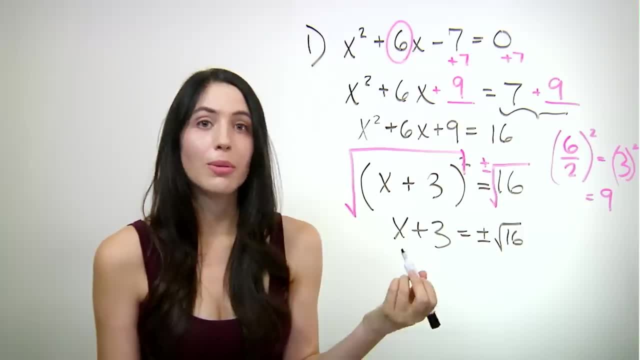 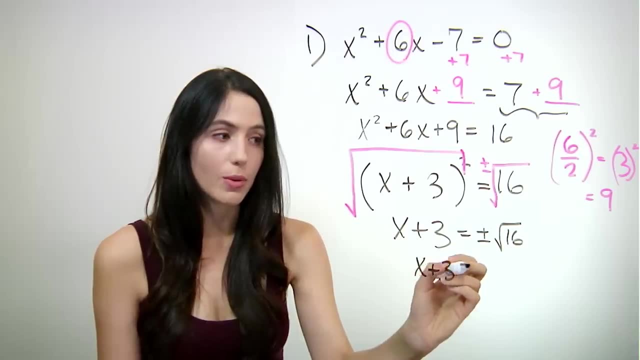 square root of 16.. You probably know, square root of 16 is 4,, since 16 is a perfect square. So then in the next line, you can write: x plus 3 equals plus and minus 4.. Okay, Okay. 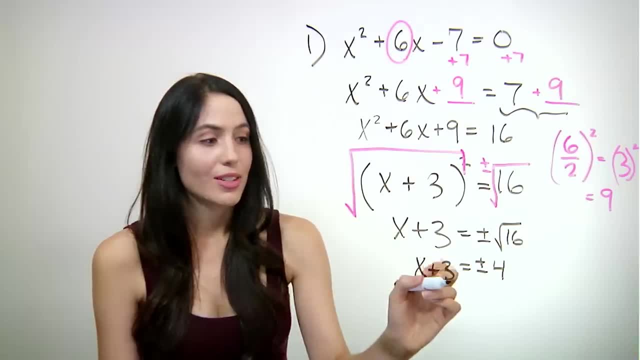 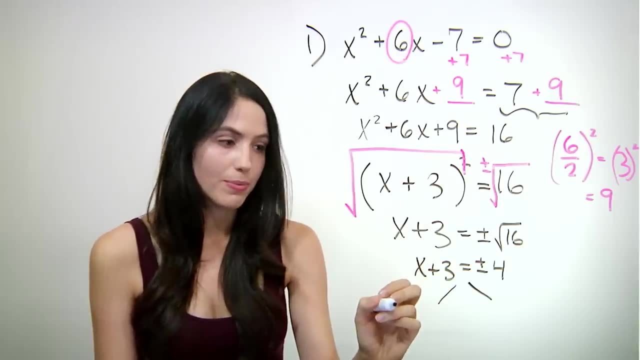 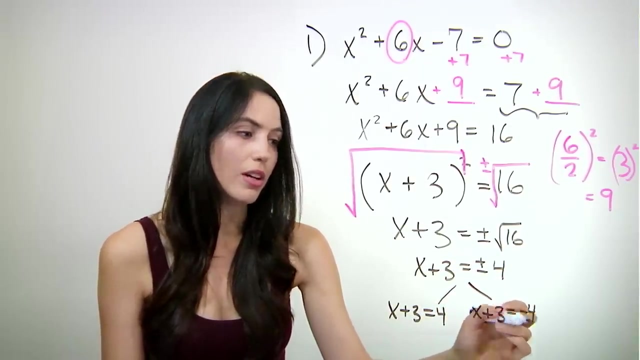 The easiest thing now is to separate this into two solutions. You're going to solve for two different answers. One equation you can write using the positive version, so x plus 3 equals 4, and the other one you'll use the negative 4 version: x plus 3 equals negative 4.. 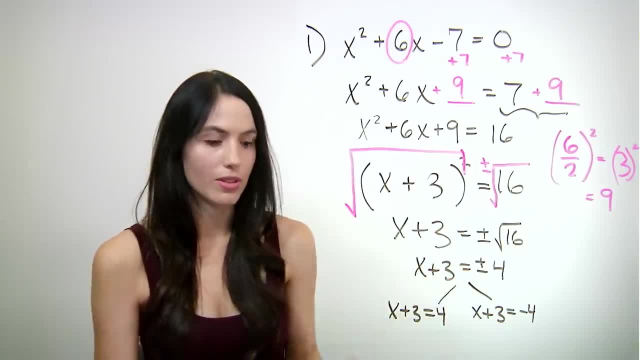 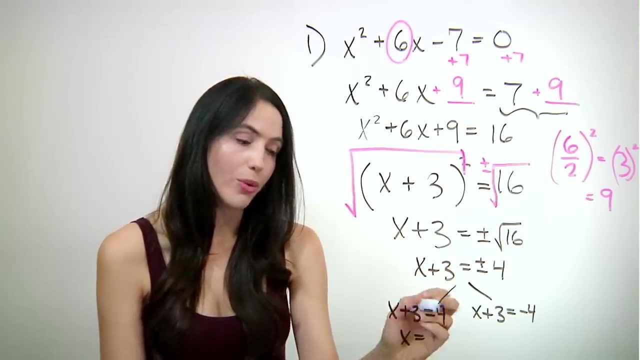 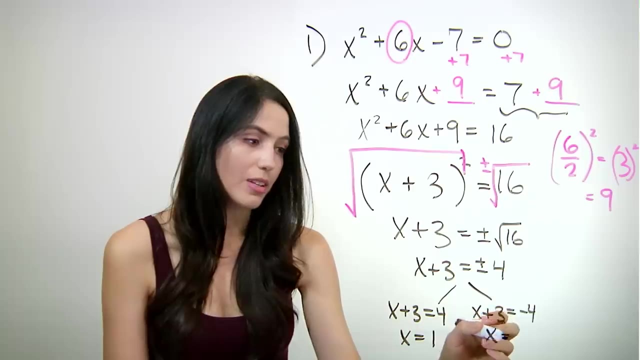 It's very important to separate it out because you will end up with two solutions. So what this gives you, Using basic algebra, subtracting constants, is: x equals 4 minus 3, or positive 1.. And on this side, x equals negative 4 minus 3,, which is negative 7.. 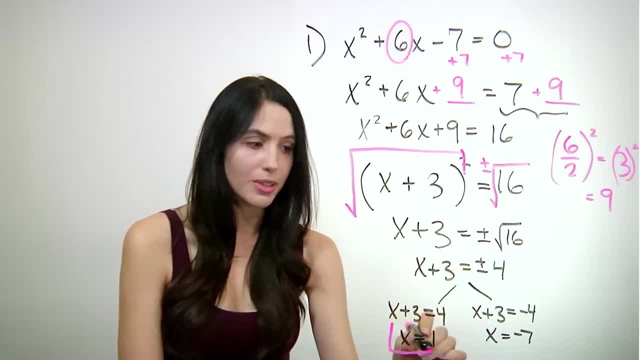 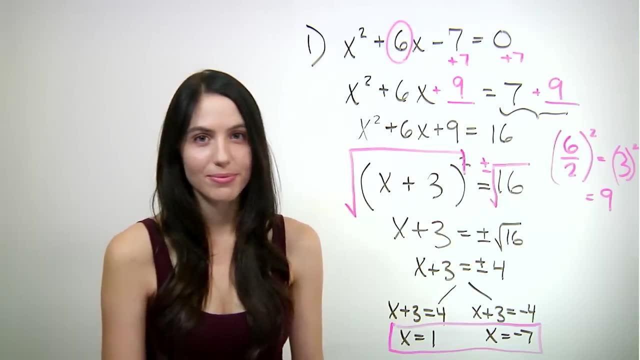 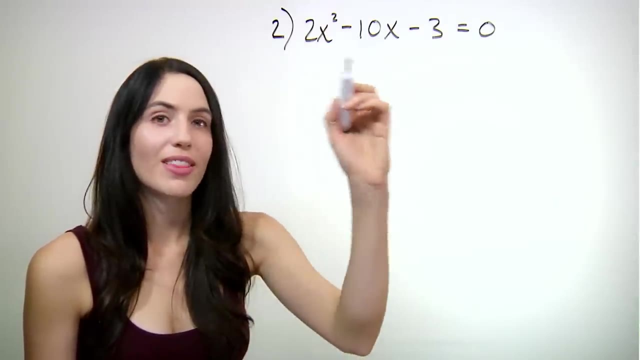 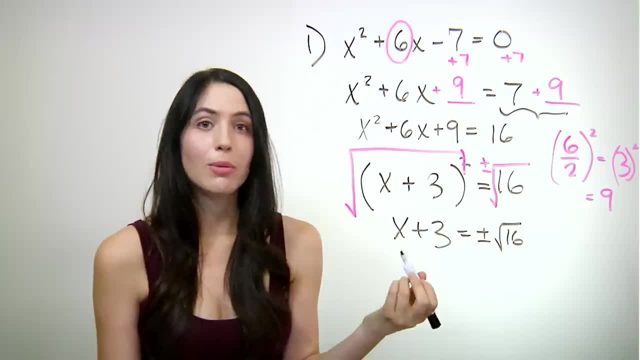 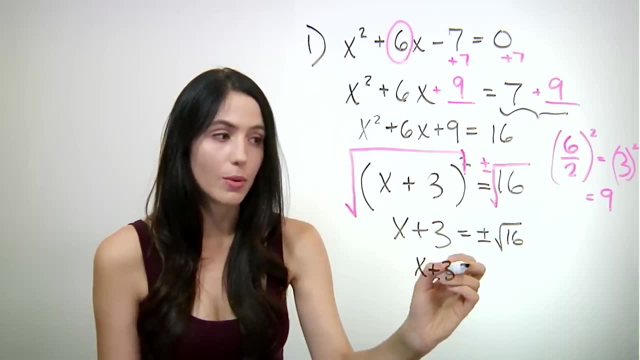 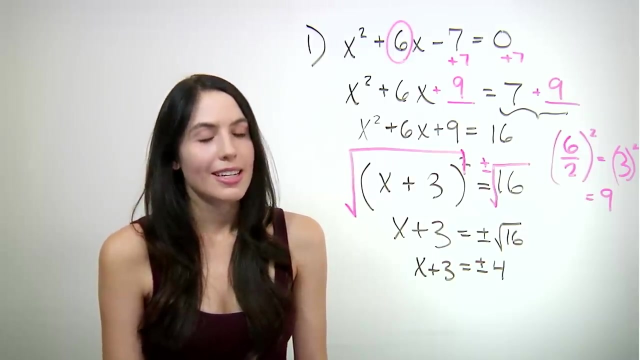 square root of 16.. You probably know, square root of 16 is 4,, since 16 is a perfect square. So then in the next line, you can write: x plus 3 equals plus and minus 4.. The easiest thing now is to separate this into two solutions. You're going to have: 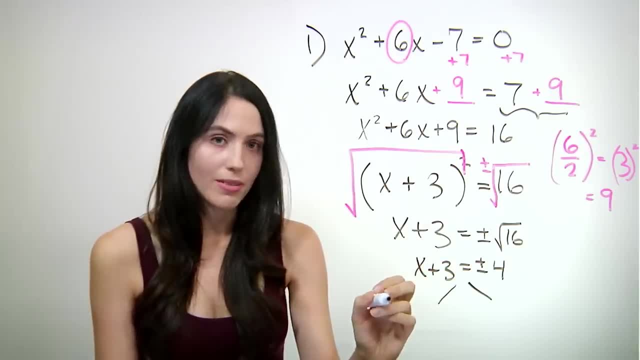 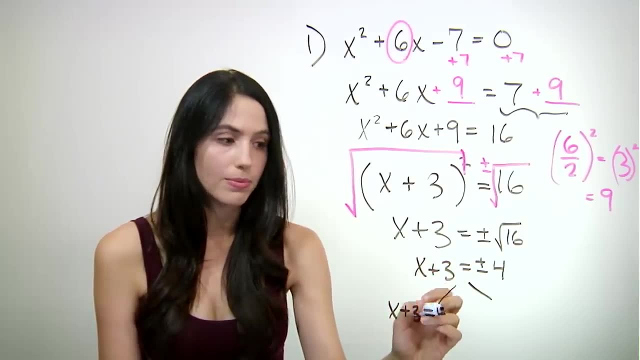 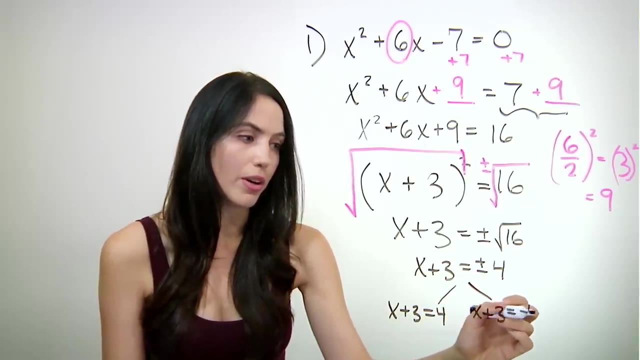 to solve for two different answers. One equation you can write using the positive version, So x plus 3 equals 4.. And the other one you'll use the negative 4 version: x plus 3 equals negative 4.. It's very important to separate it out because you will end up with two solutions. 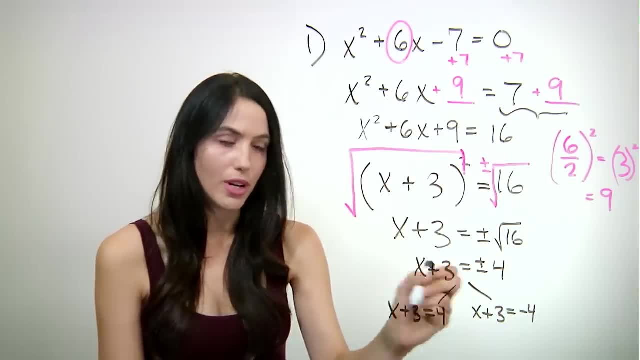 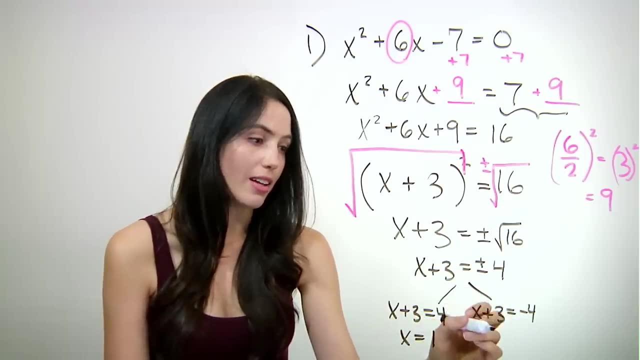 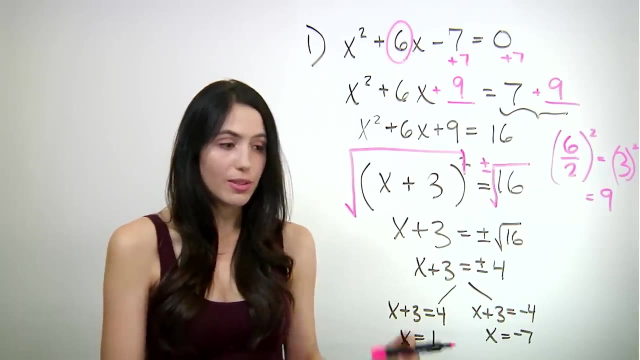 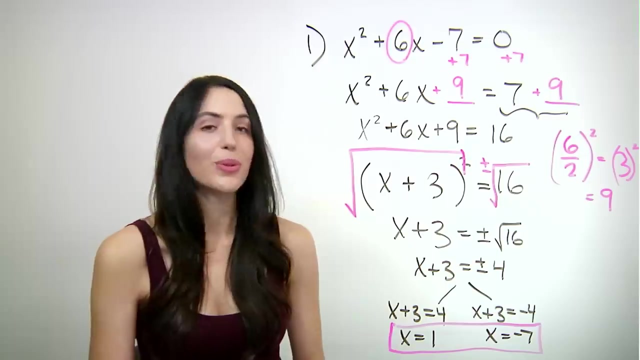 So what this gives you, using basic algebra, subtracting constants, is x equals 4 minus 3.. And on this side, x equals negative 4 minus 3, which is negative 7.. So your two solutions using completing the square are x equals 1 and x equals negative 7.. 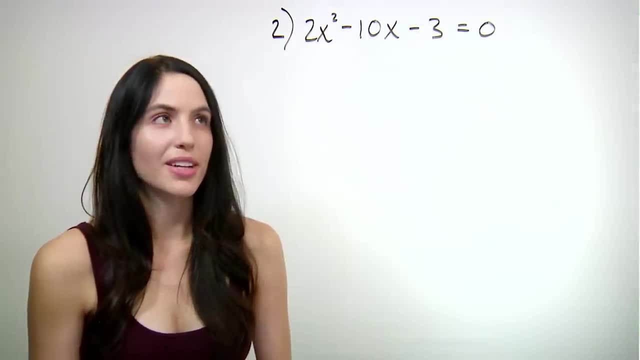 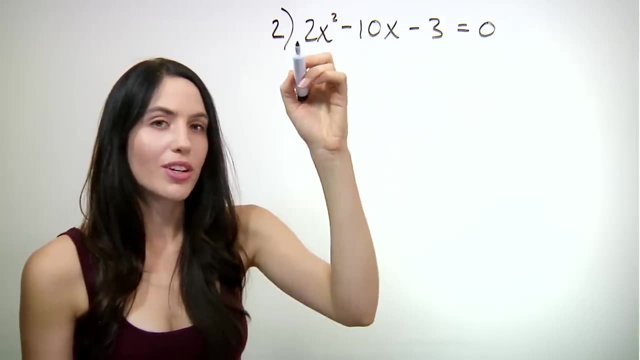 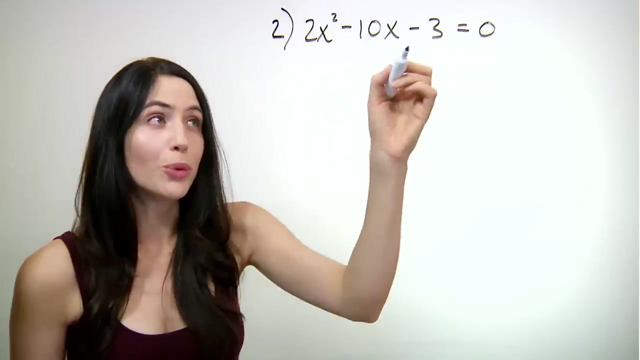 Okay, Say you have an equation that looks like this: with 2x squared or 3x squared, where the coefficient of x squared is something bigger than 1.. The first step will be the same: You're going to move this constant to the right side. So, since it's minus 3, right? 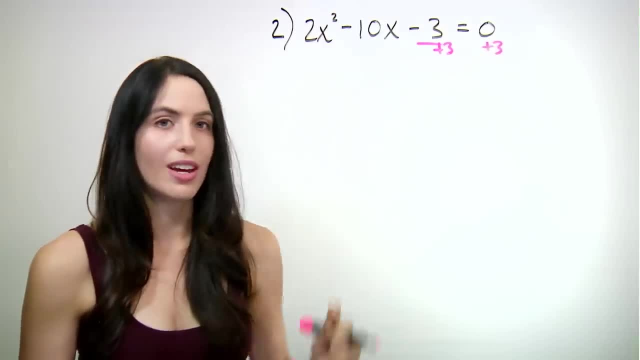 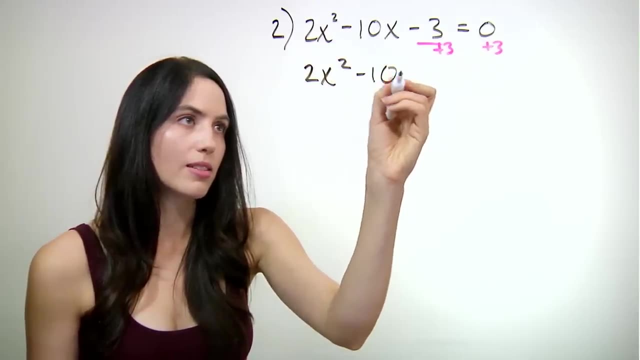 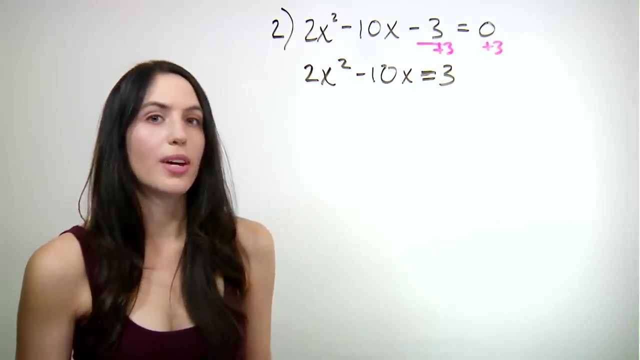 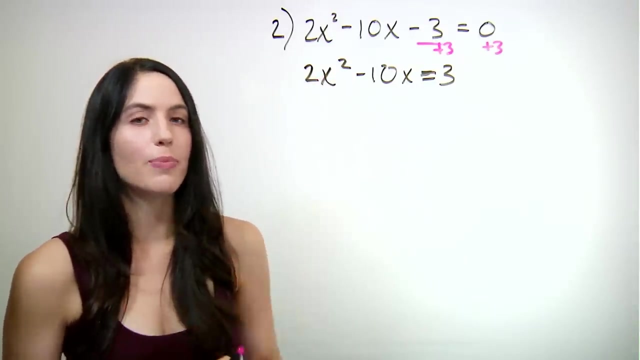 now you can add 3 to both sides in order to move it to the right, And you get 2x squared minus 10x equals positive 3.. Now what you have to do? because there is a 2 attached to the x squared, or 3, or 4, etc. 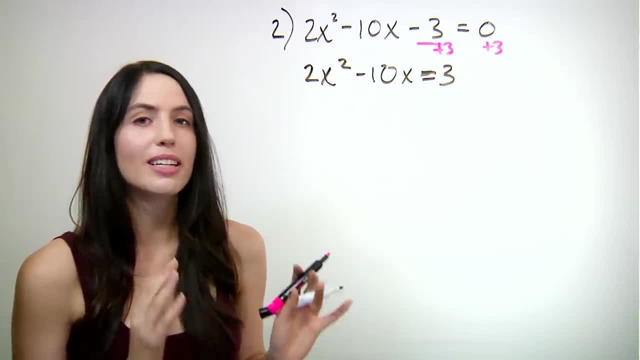 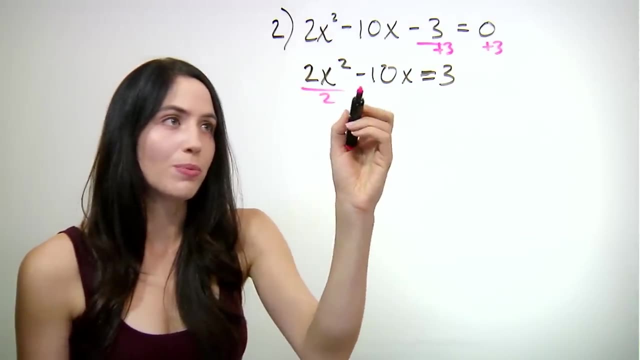 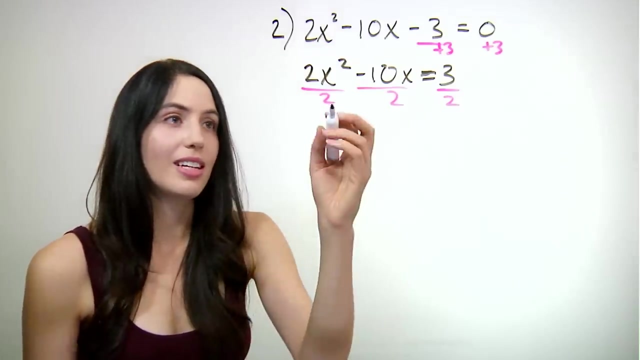 You have to divide it out from every term in the equation. That will make it easier for you to complete the square. It will make it possible for you to complete the square. So you're dividing every term by 2.. That includes the right hand side. So what you get is just 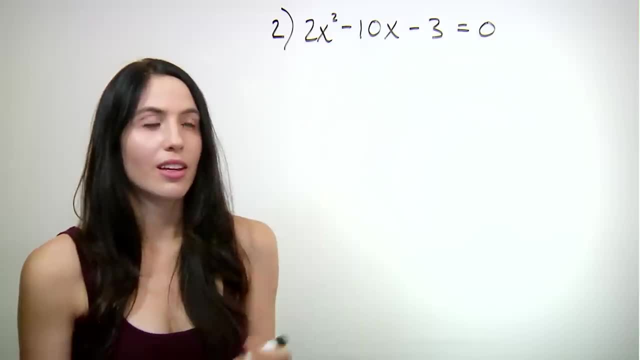 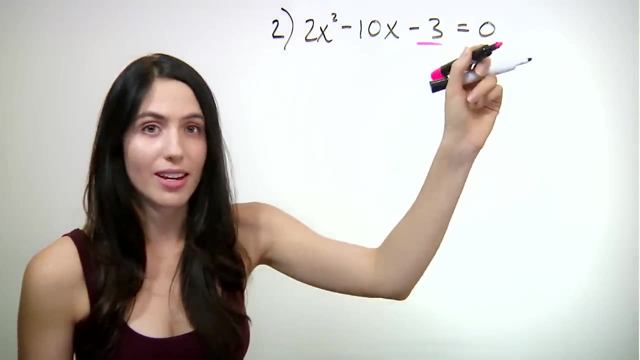 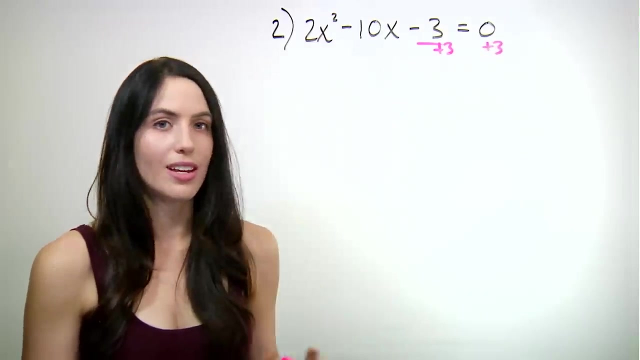 where the coefficient of x squared is something bigger than 1.. The first step will be the same: You're going to move this constant to the right side. So, since it's minus 3 right now, you can add 3 to both sides in order to move it to the. 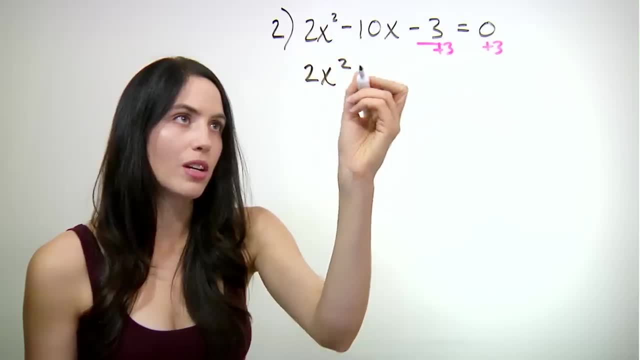 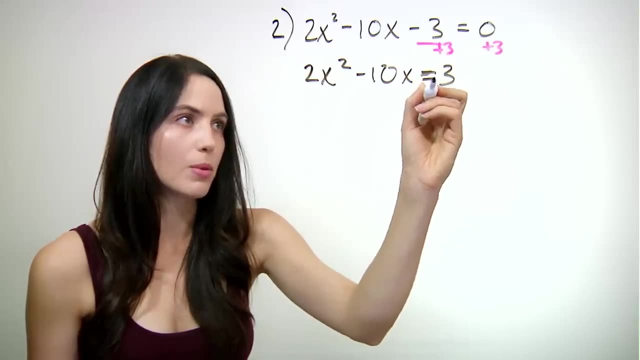 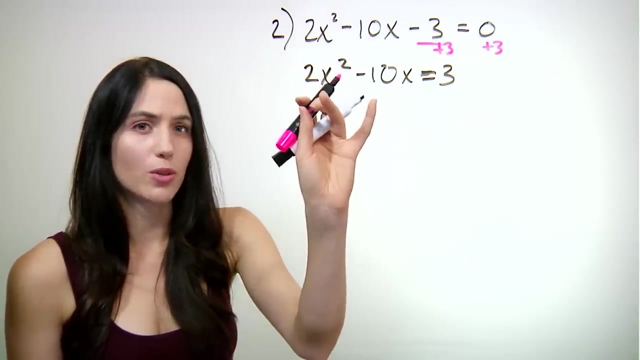 right. 2x squared minus 10x equals positive 3, equals positive 3.. Okay, now what you have to do? because there is a 2 attached to the x squared, or 3 or 4, etc. you have to divide it out from every term in the equation. 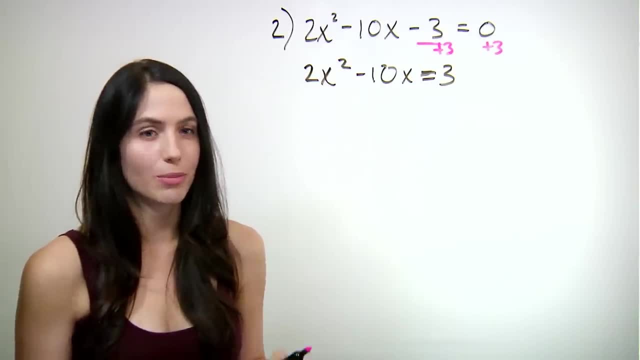 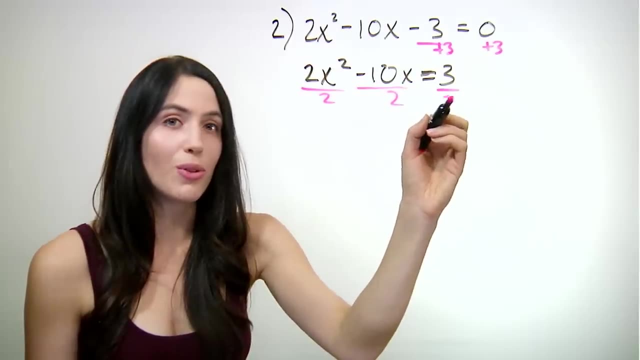 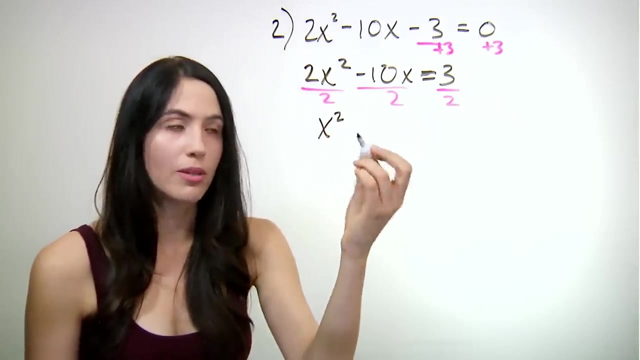 That will make it easier for you to complete the square. It will make it possible for you to complete the square. So you're dividing every term by 2. That includes the right-hand side. So what you get is just x squared now, which isn't good. 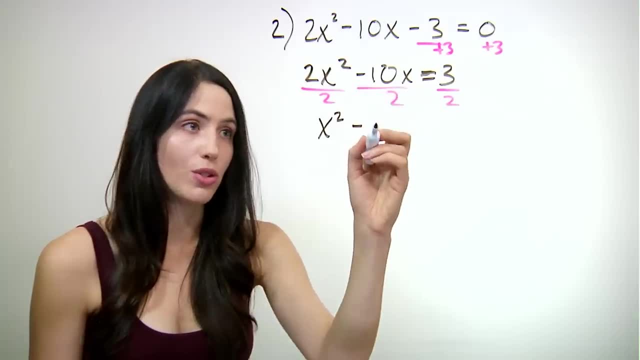 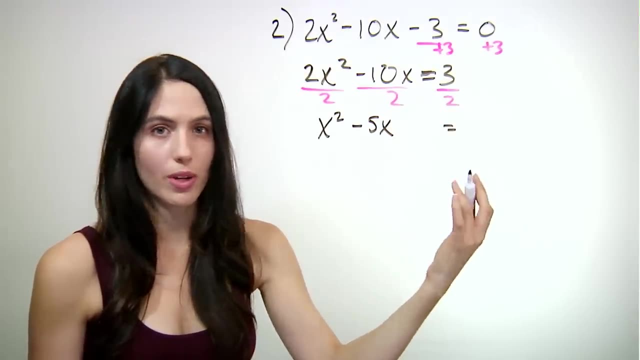 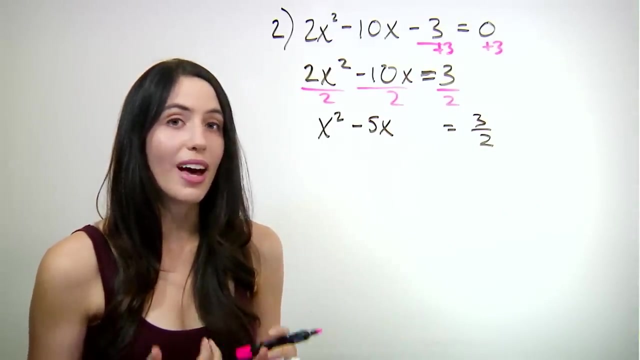 minus 5x, since it was negative, 10x over 2.. And on the right side you have 3 divided by 2, which is already in simplest form. It's just 3 halves on the right side. The next step is to add a number to both sides. 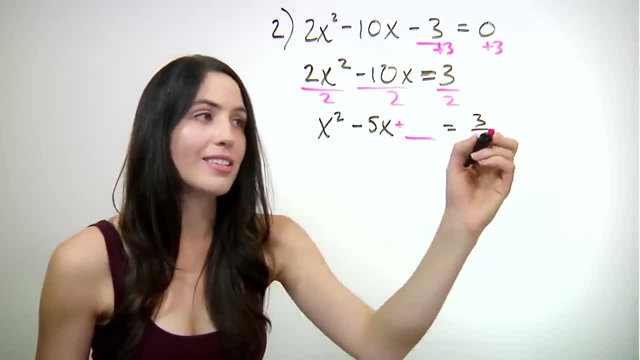 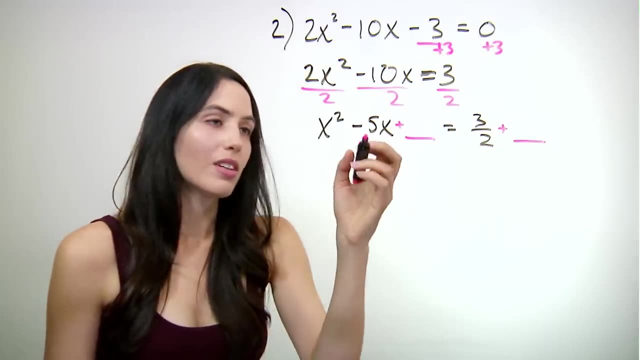 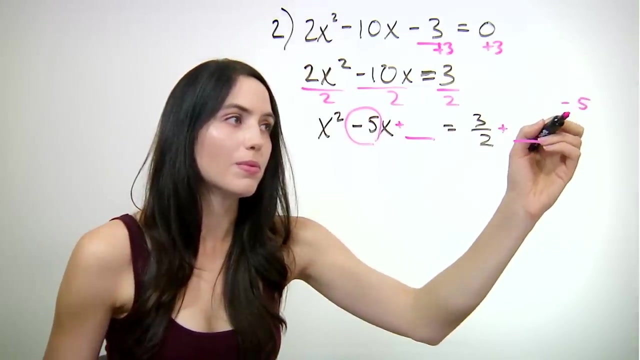 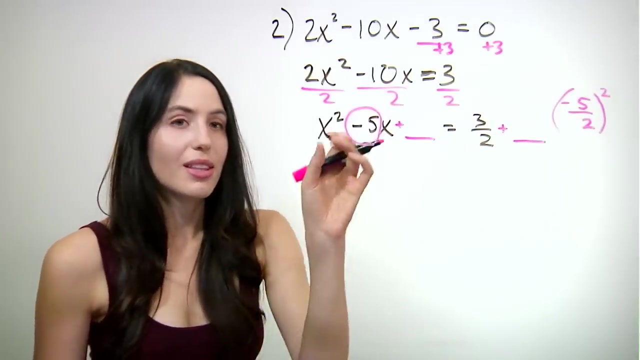 So you're going to add something here and the same something here. What number do you add? You add this coefficient of x, but divided by 2 and squared. So it's always So, it's always The coefficient of x over 2, then squared. 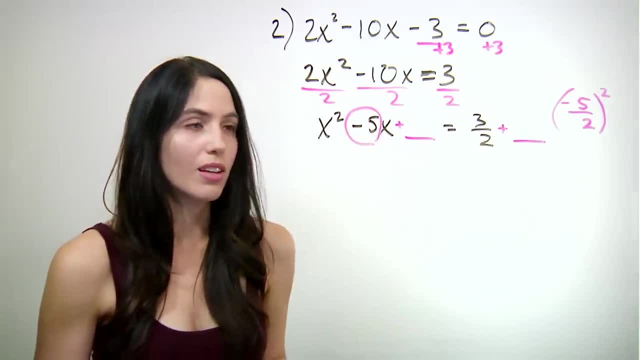 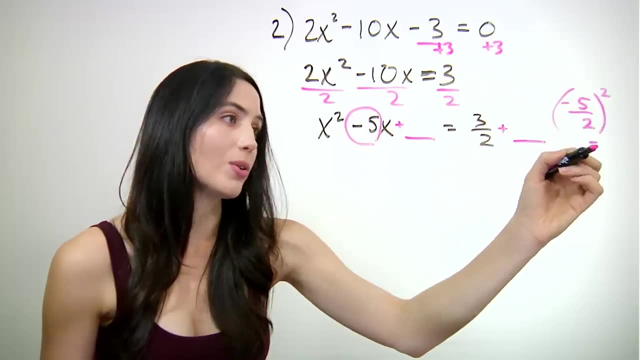 and that is what you add to the left side and the right side. So in this problem that's negative 5 divided by 2, all squared, which simplifies to positive 25, because negative 5 times negative 5 is positive 25,. 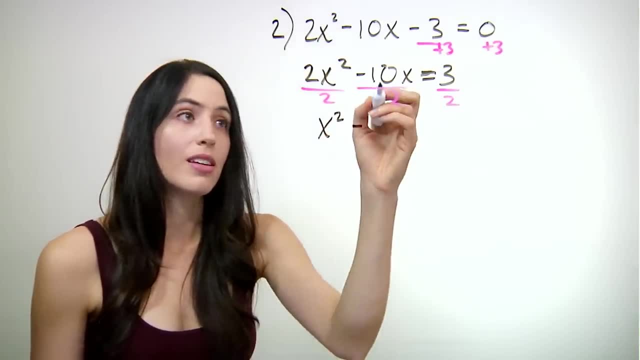 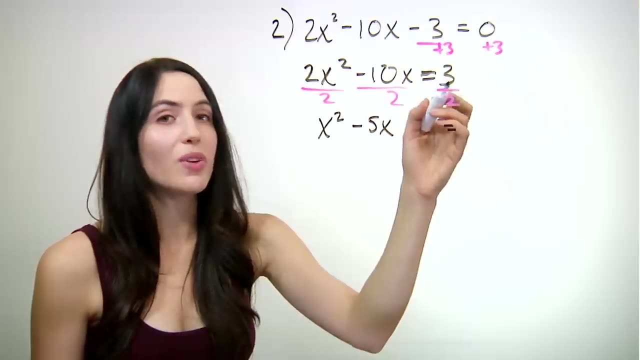 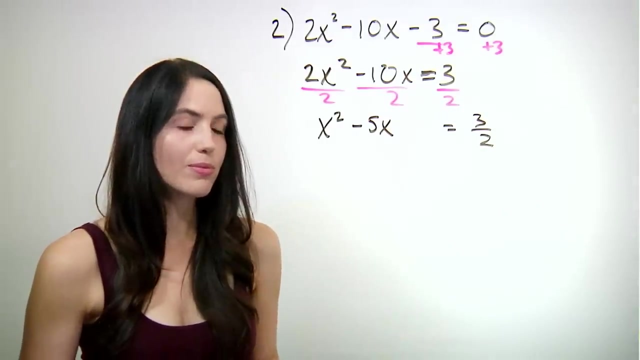 x squared now, which is good, minus 5x, since it was negative- 10x over 2.. And on the right side you have 3 divided by 2, which is already in simplest form. It's just 3 halves on the right side. 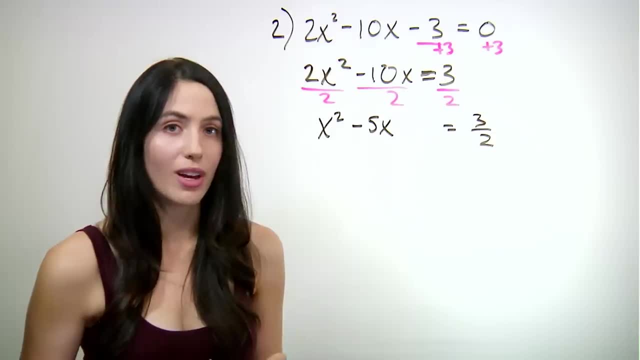 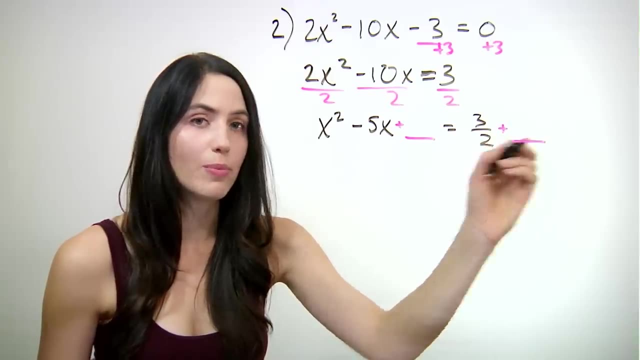 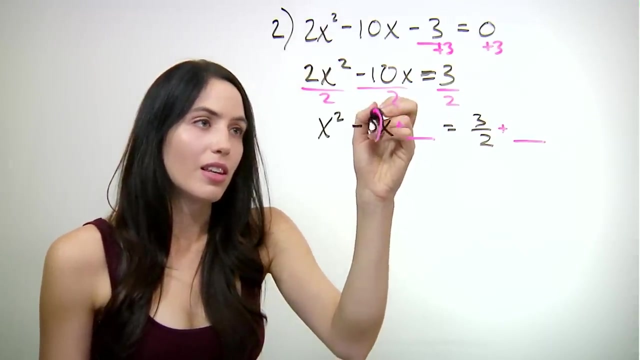 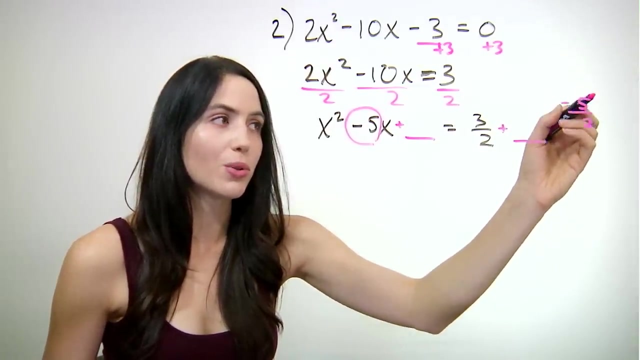 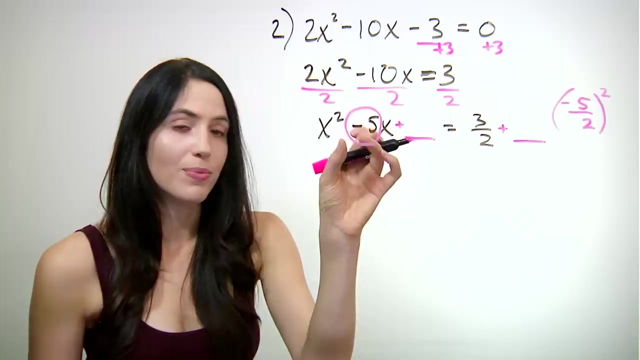 The next step is to add a number to both sides. You're going to add something here and the same something here. What number do you add? You add this coefficient of x, but divided by 2 and squared, So it's always the coefficient of x over 2, then squared. 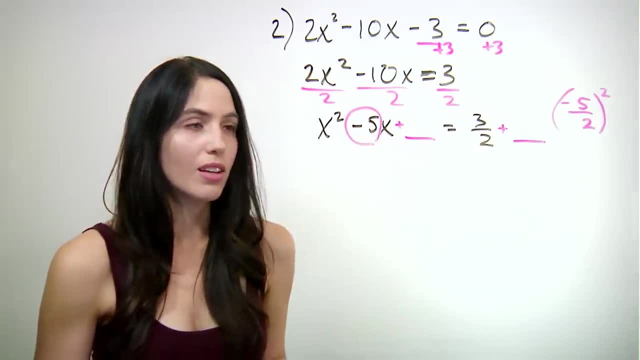 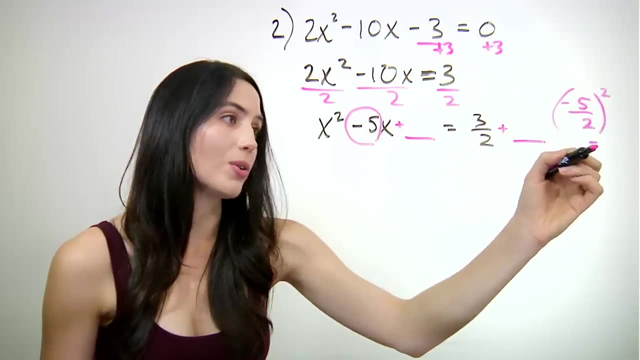 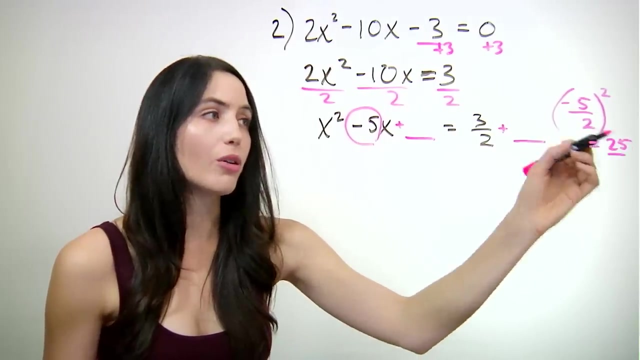 and that is what you add to the left side and the right side. So in this problem that's negative 5 divided by 2. All squared, which simplifies to positive 25, because negative 5 times negative 5 is positive 25,. 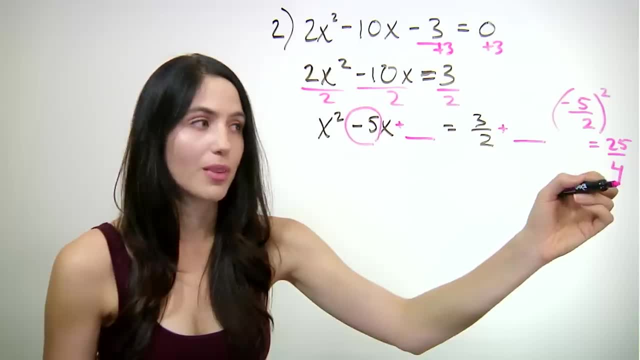 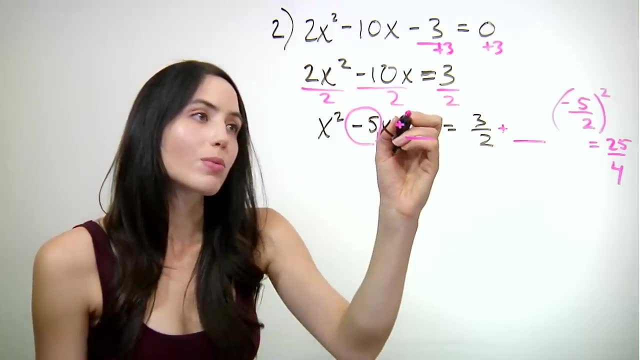 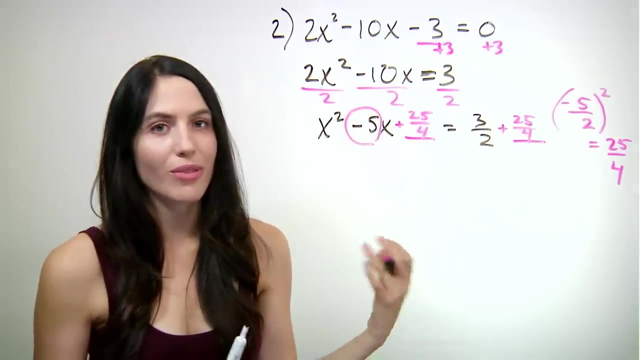 over 2 squared on the bottom, which is 4.. So you're adding the fraction 25 over 4 to both sides. I gave you one that has a fraction because a lot of times completing the square problems end up a little ugly. 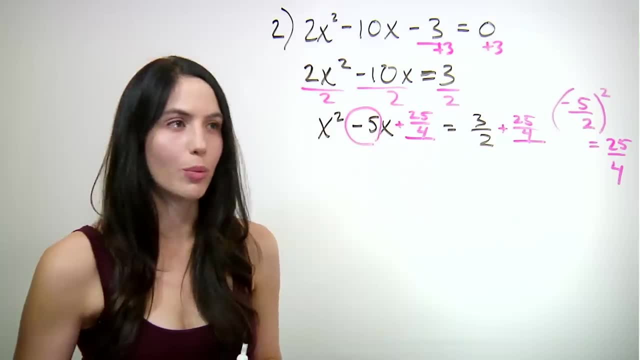 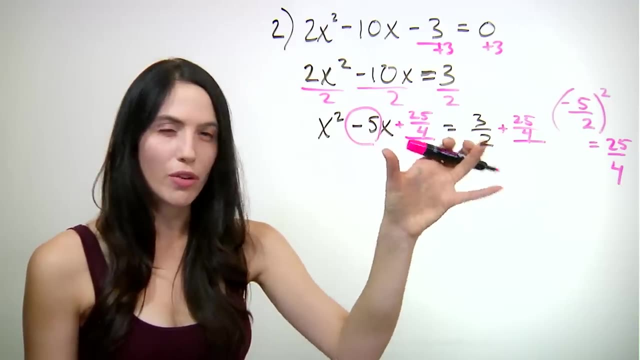 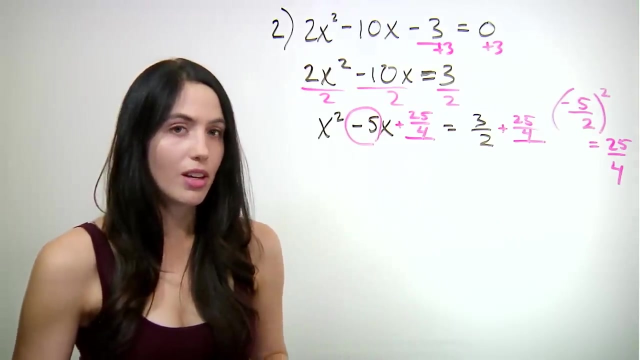 and have fractions involved, So you'll probably have one like that in your homework. Now you added the same number to both sides because you don't want to change the overall value of the equation. You want to keep it balanced, And what this lets you do immediately after is write. 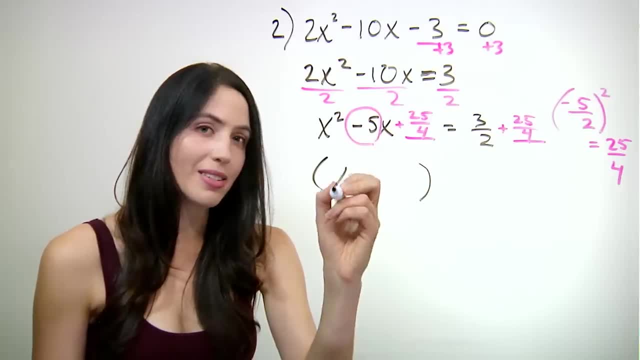 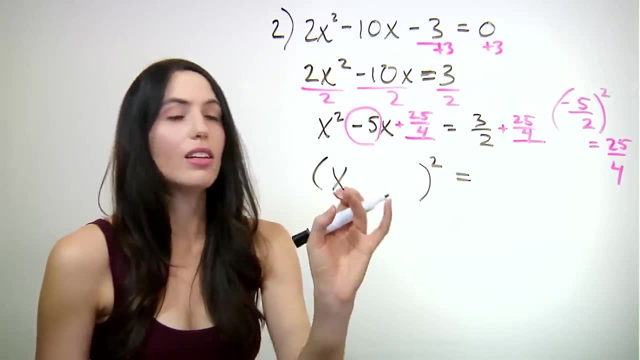 the left-hand side as a perfect square, meaning x plus or minus a number squared. That's the whole point. The point of adding that number is so that on the left side you can immediately write x and some number here squared. What number do you write? 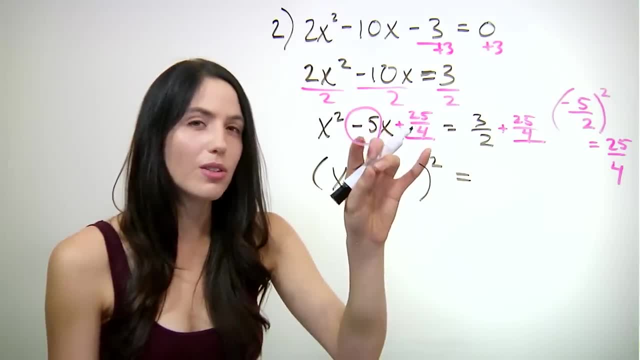 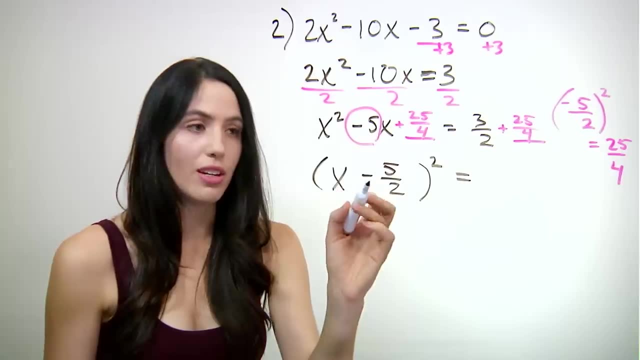 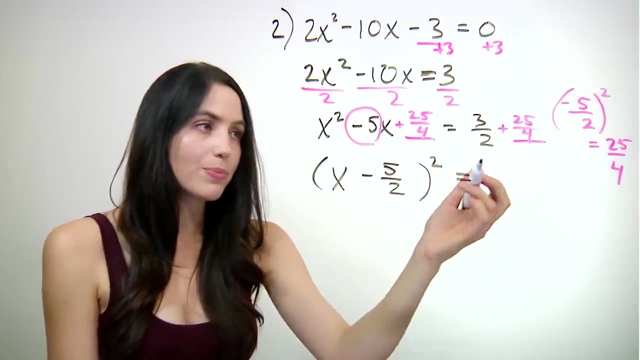 It's this coefficient over 2.. So it's negative 5 over 2.. And since it's negative, instead of addition it's subtraction minus. 5 over 2 squared equals the right-hand constant. Since this is an uglier example, 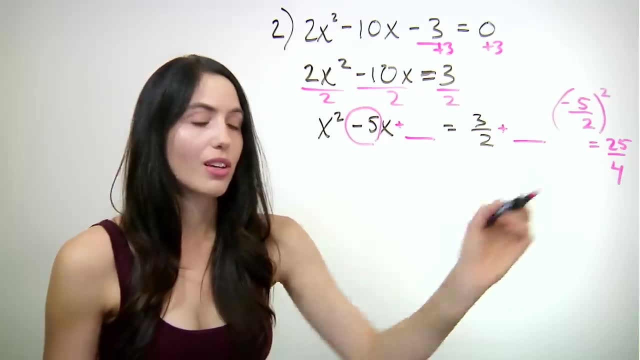 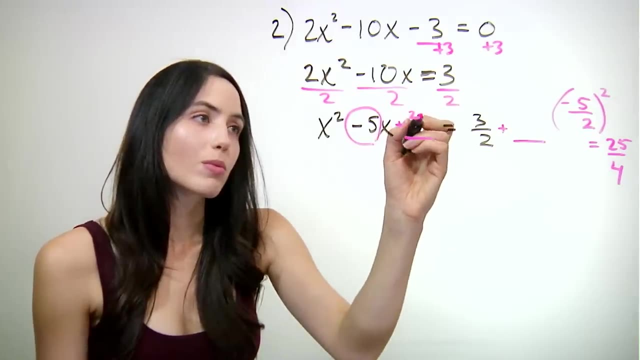 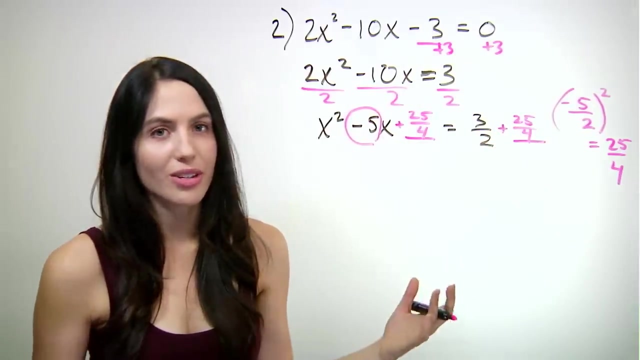 over 2 squared on the bottom, which is 4.. So you're adding the fraction 25 over 4, to both sides. I gave you one that has a fraction because a lot of times completing the square problems end up a little ugly and have fractions involved. 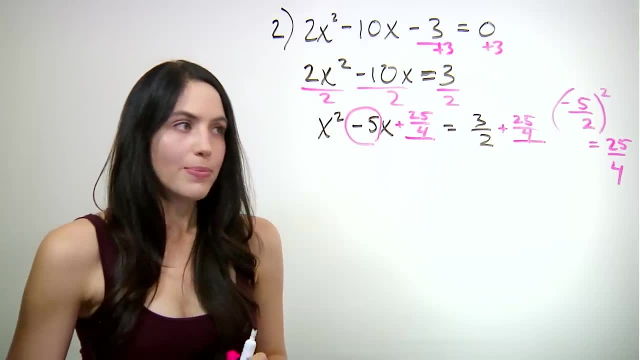 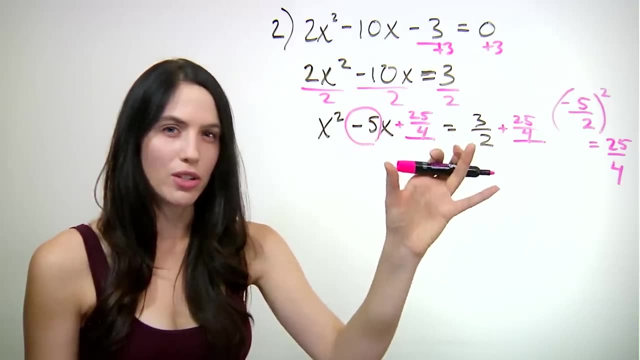 So you'll probably have one like that in your homework. Now you added the same number to both sides because you don't want to change the overall value of the equation. You want to keep it balanced, And what this lets you do immediately after. 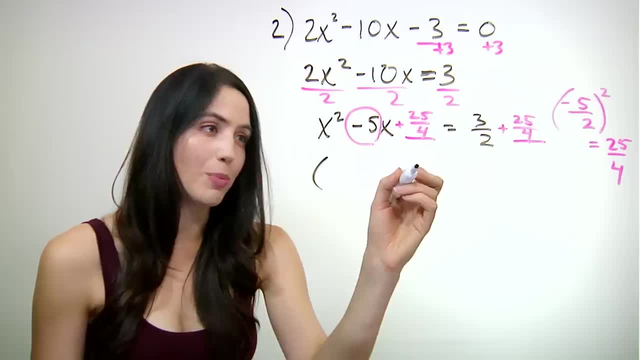 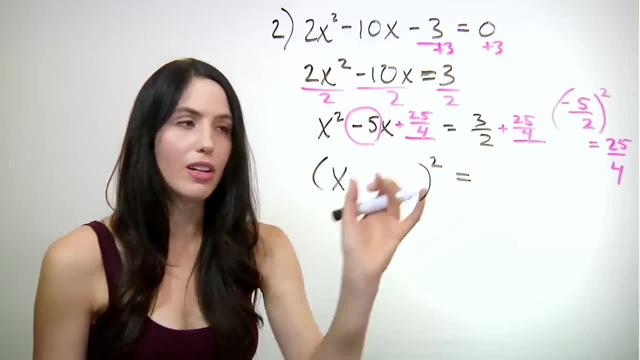 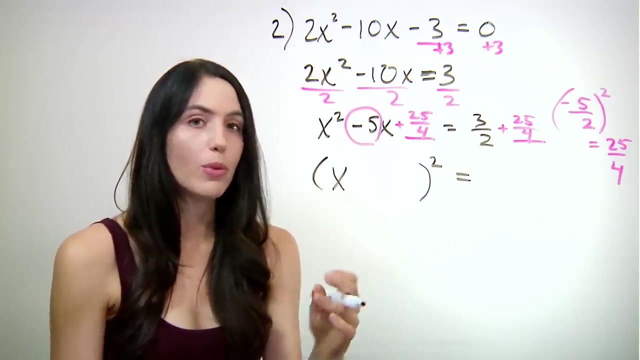 is write the left-hand side as a perfect square, meaning x plus or minus a number squared. That's the whole point of adding that number is so that on the left side you can immediately write x and some number here squared. What number do you write? 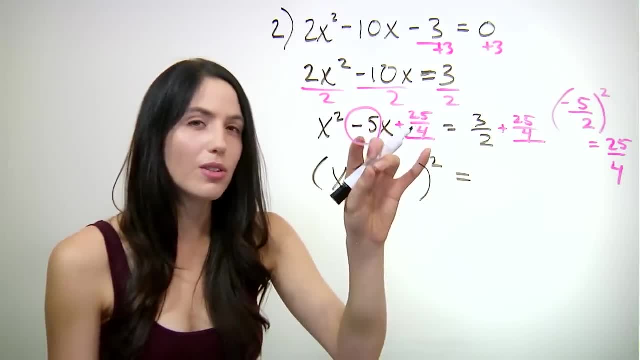 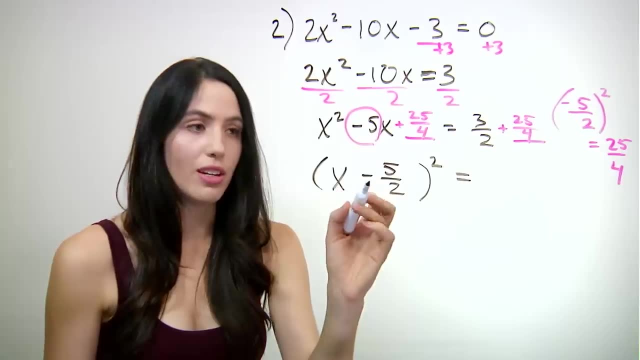 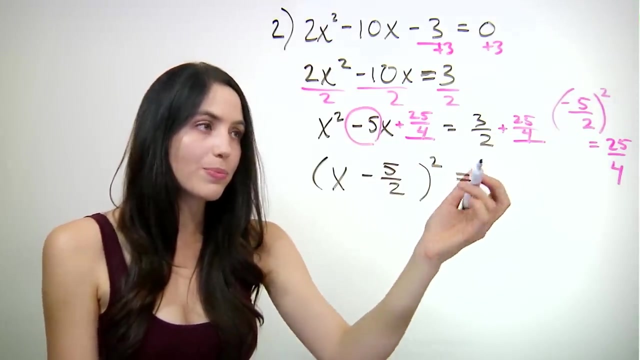 It's this coefficient over 2.. So it's negative: 5 over 2.. And since it's negative, instead of addition it's subtraction minus 5 over 2, squared equals the right-hand constant. Since this is an uglier example, it has some fractions involved. 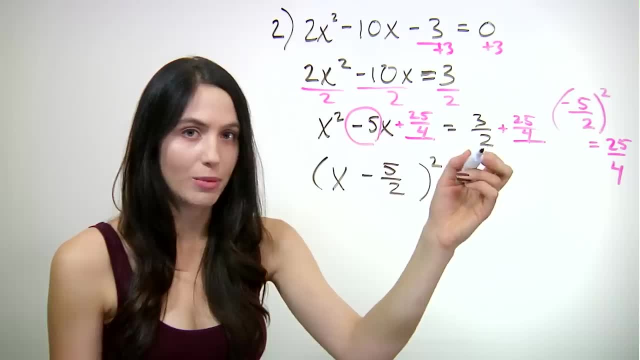 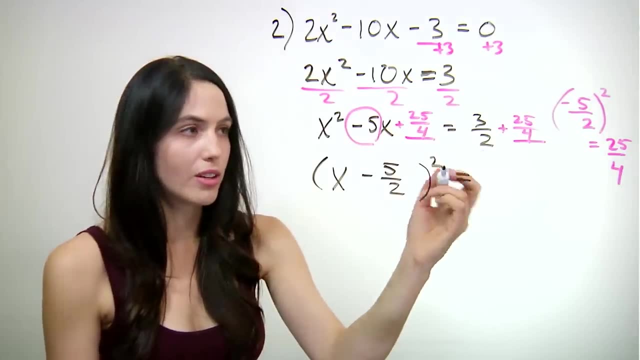 You'll have to get a common denominator in order to combine them or plug them into your calculator. if you're allowed to use your calculator, A lot of calculators are very good at adding and simplifying fractions. What you have to do is get a common denominator. 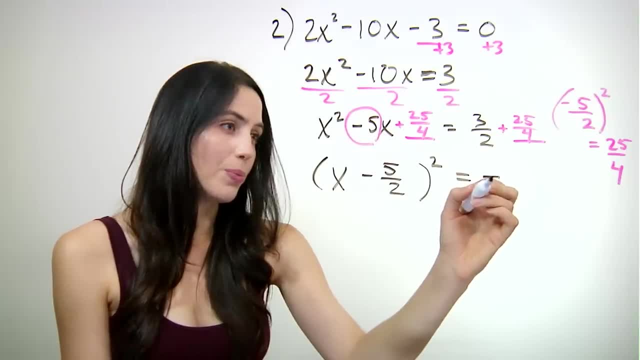 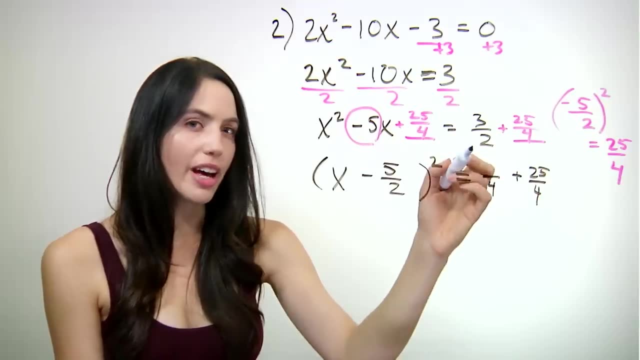 which would be 4 in this case. So you have 25 over 4, and you have 3 halves, which can also be written as 6 over 4.. If you multiply the bottom by 2 to get 4,. 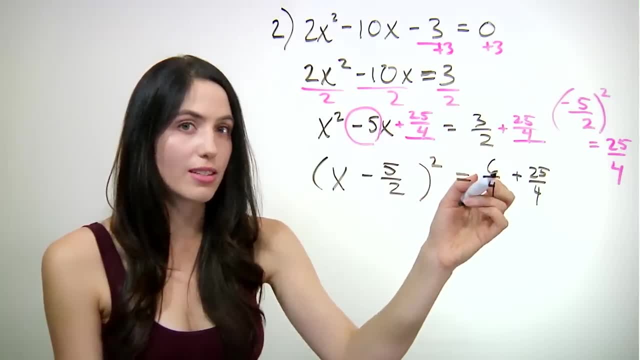 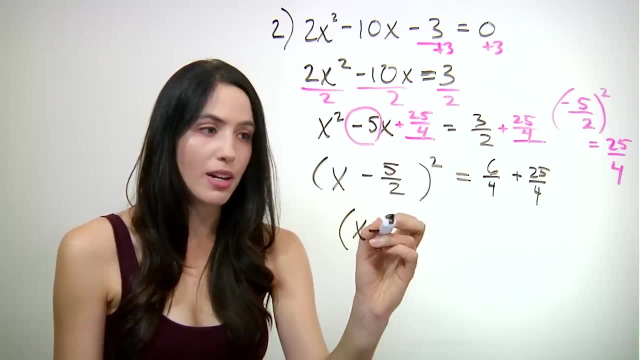 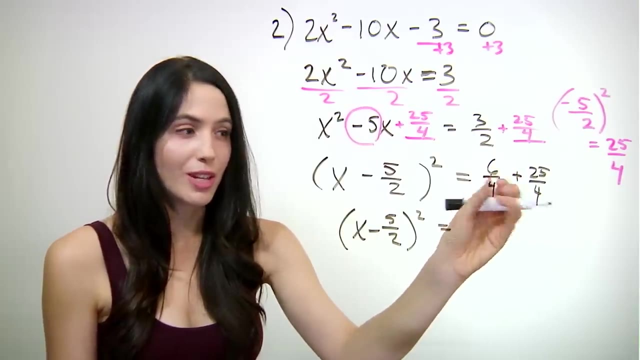 you also have to multiply the top by 2 to get 6.. So in the next line you can rewrite this as x minus 5, halves squared equals, and combine the fractions. Since the denominators are the same, you keep it as 4,. 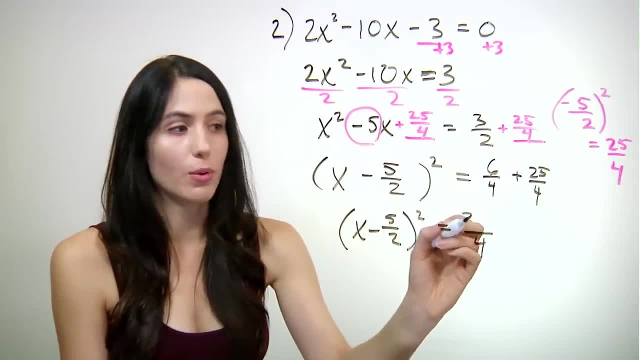 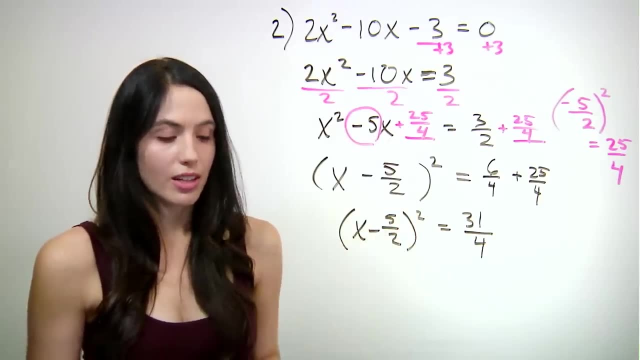 and the numerators you add. So 6 plus 25 gives you 31.. Great, so you've completed the square, And this is in a form that will be very easy for you to solve. What you want to do is square roots both sides. 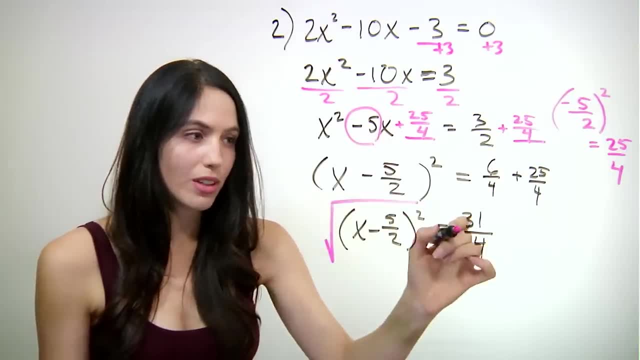 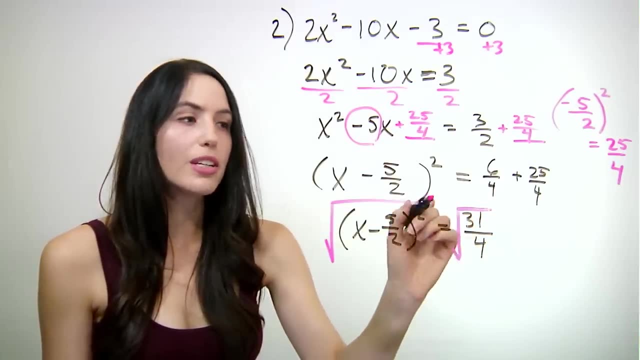 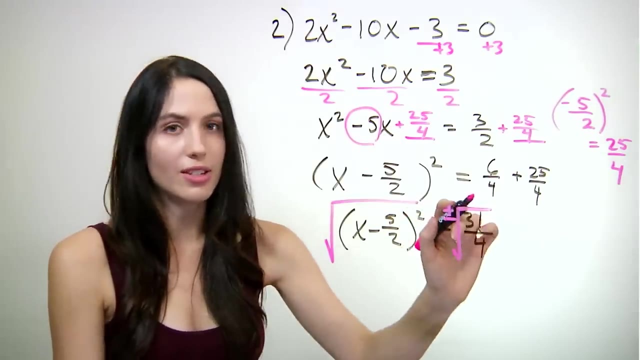 So on the left side it's a big square root. On the right side you do a square root of the constant but you immediately get positive and negative versions. So remember, when you square root this side, that is just a number. 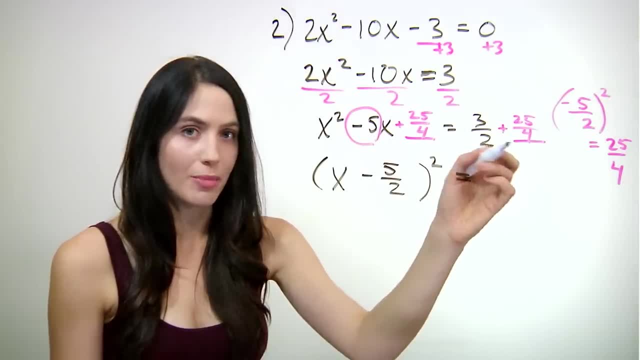 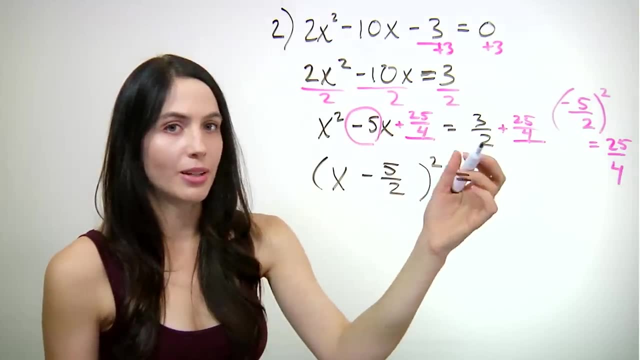 it has some fractions involved. You'll have to get a common denominator in order to combine them Or plug them into your calculator. if you're allowed to use your calculator, A lot of calculators are very good at adding and simplifying fractions. What you have to do is get a common denominator. 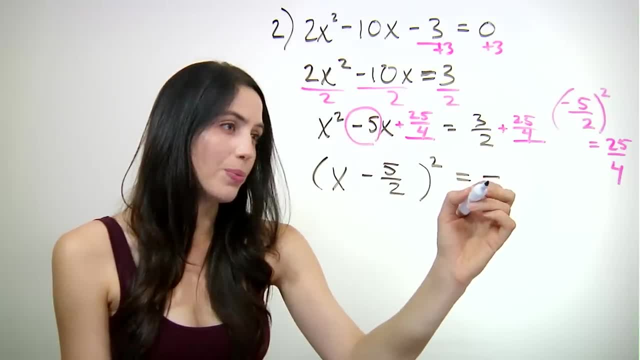 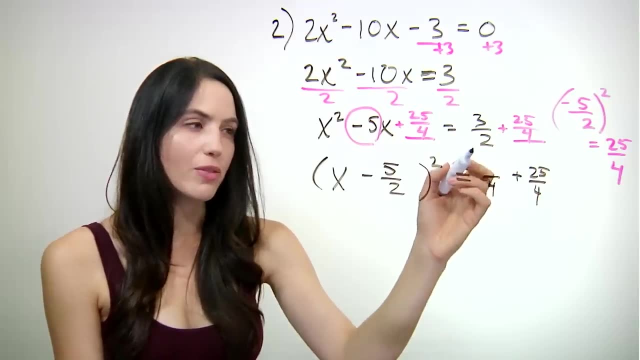 which would be 4 in this case. So you have 25 over 4, and you have 3 halves, which can also be written as 6 over 4.. You multiply the bottom by 2.. You get 4.. You also have to multiply the top by 2 to get 6.. 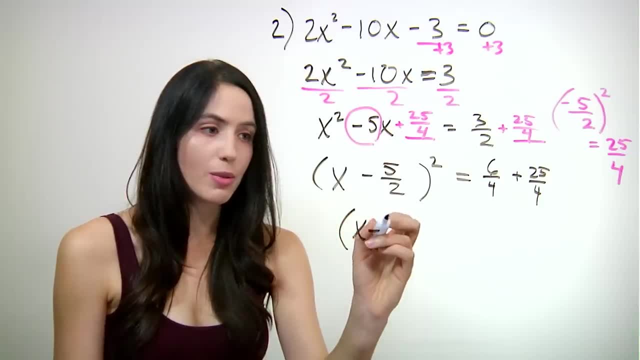 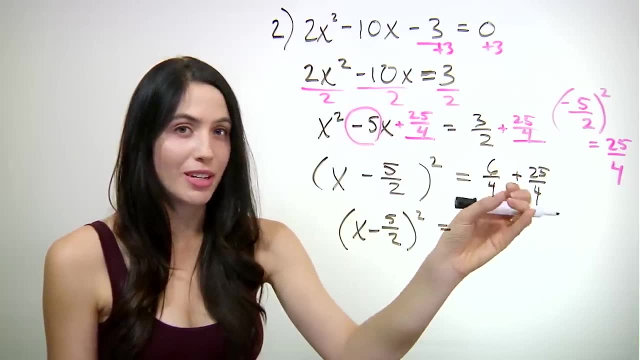 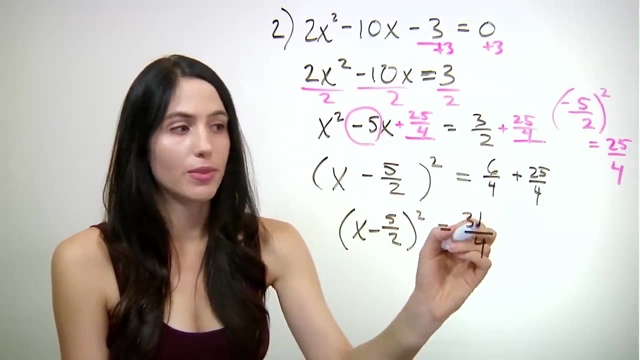 So in the next line you can rewrite this as x minus 5, halves squared equals, and combine the fractions. Since the denominators are the same, you keep it as 4, and the numerators you add. So 6 plus 25 gives you 31.. 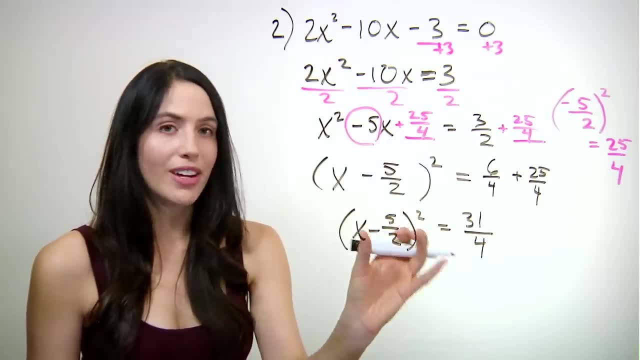 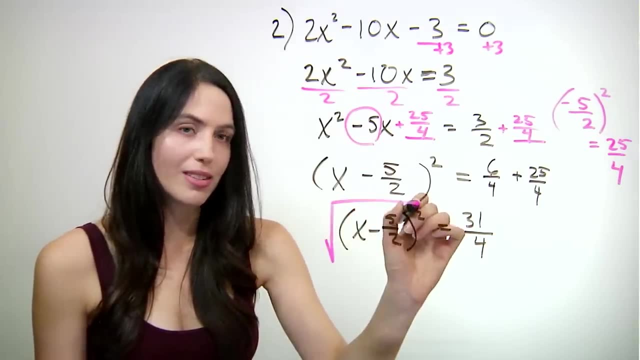 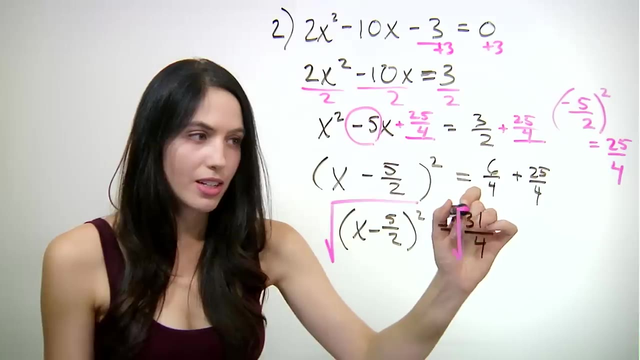 Great. so you've completed the square, And this is in a form that will be very easy for you to solve. What you want to do is square roots both sides. So on the left side it's a big square root. On the right side you do a square root of the constant. 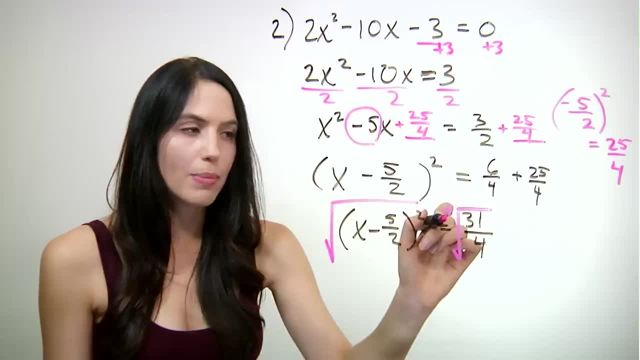 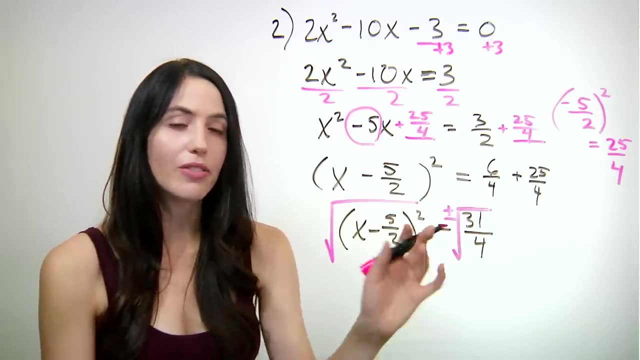 but you immediately get positive and negative versions. So remember, when you square root the side- that is just a number- you have to put plus and minus. If you don't, you'll only have half the solutions. You'll only have 1 instead of 2 solutions in the end. 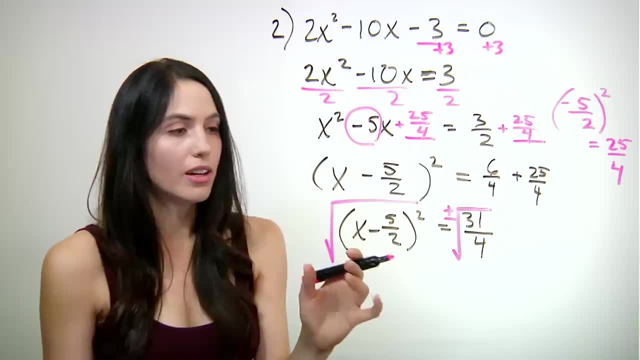 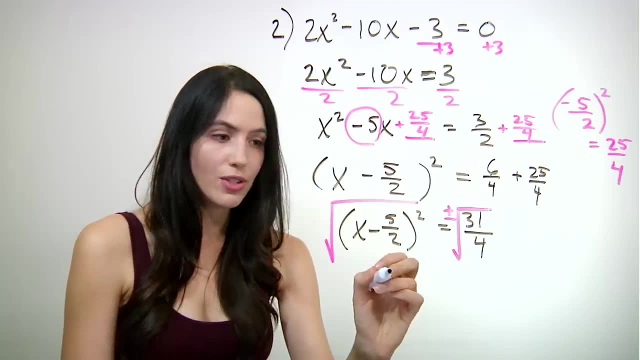 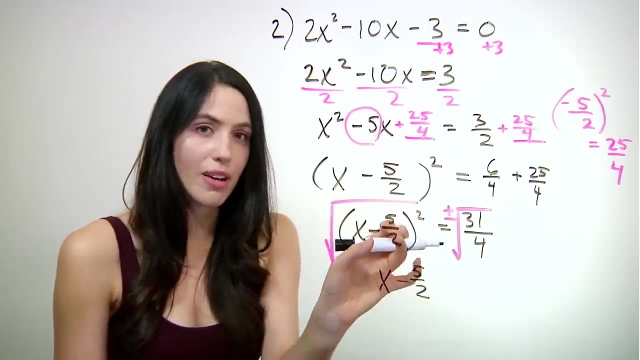 So it's very important. People forget it all the time. But you want to square root both sides. What that leaves you on the left is just x minus 5 halves, because your square root undid the square and you just have what's left inside the parentheses. 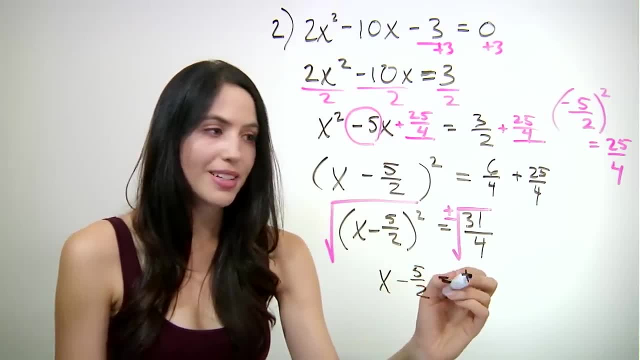 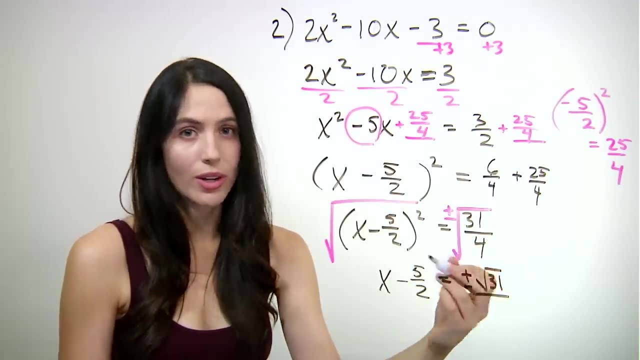 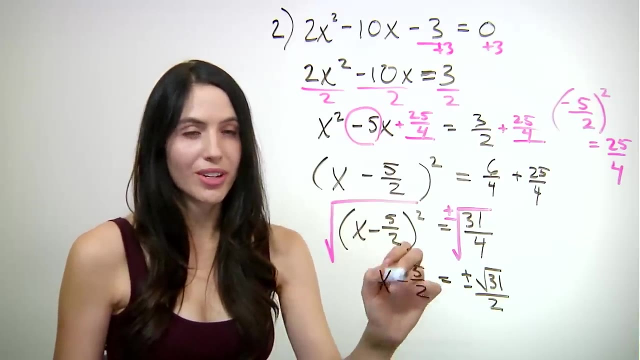 So x minus 5 halves equals plus and minus square root of 31.. Over square root of 4, which you can just write as 2. Then you'll want to use some simple algebra to move this constant over. so you have x alone. 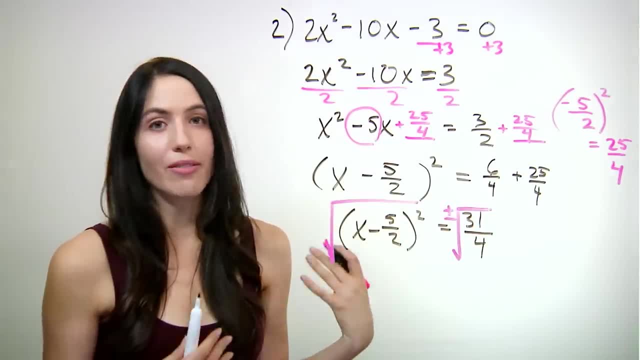 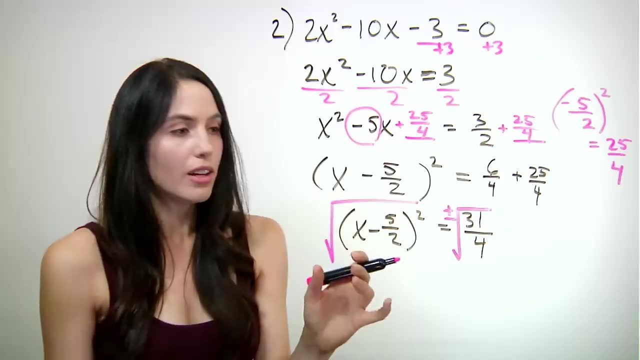 you have to put plus and minus. If you don't, you'll only have half the solutions. You'll only have 1 instead of 2 solutions in the end. So it's very important. People forget it all the time. But you want to square root both sides. 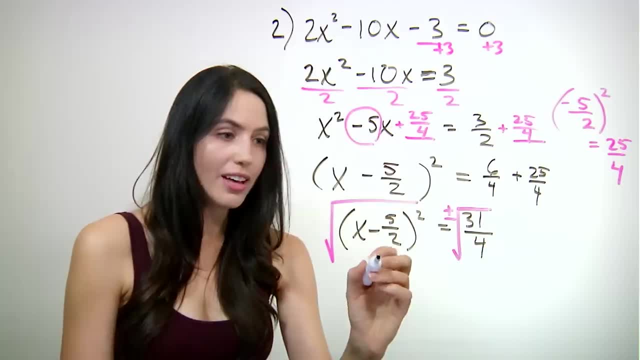 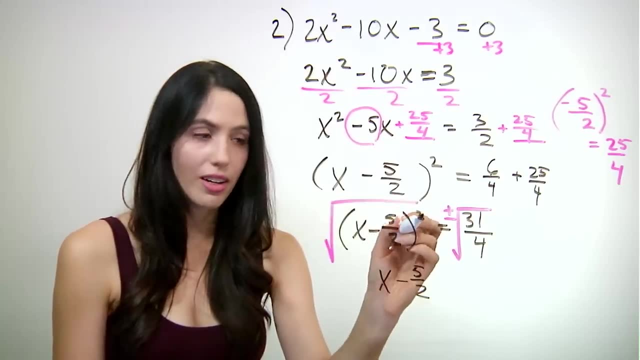 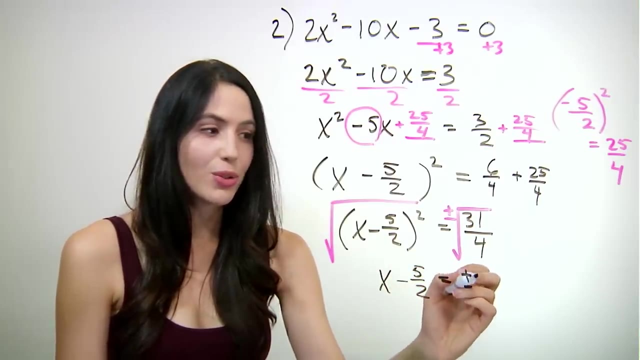 What that leaves you on the left is just x minus 5 halves, because your square root undid the square and you just have what's left inside the parentheses. So x minus 5 halves equals plus and minus square root of 31 over square root of 4,. 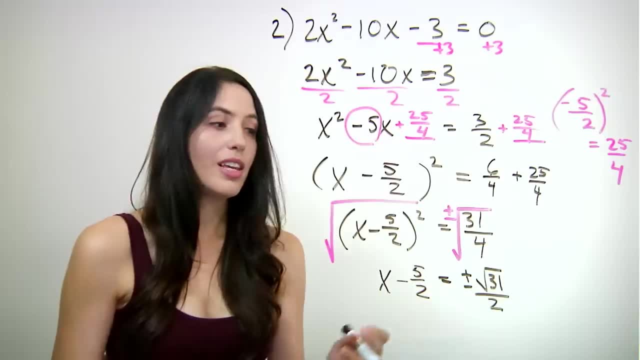 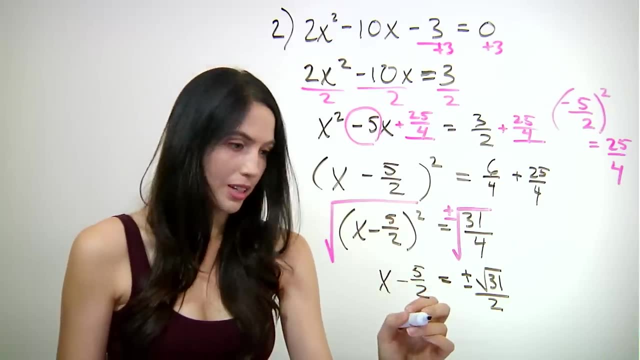 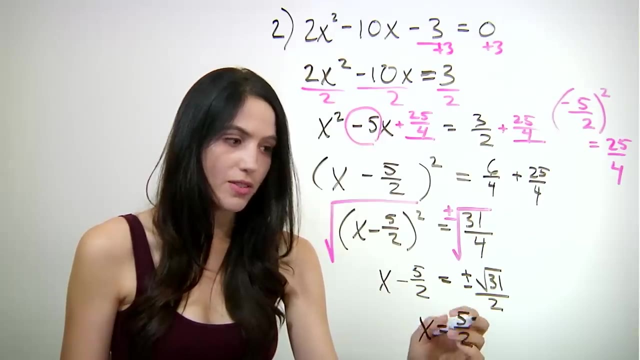 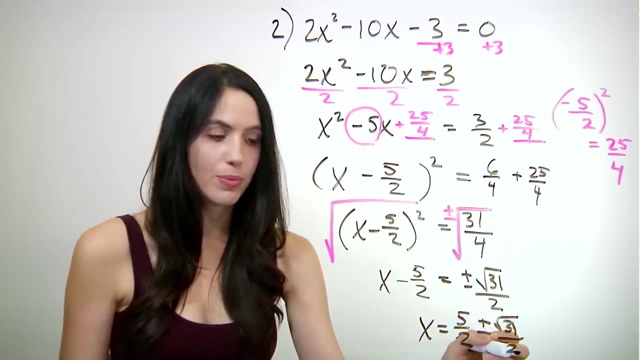 which you can just write as 2.. Then you'll want to use some simple algebra to move this constant over. so you have x alone And your two solutions will be: x equals 5 halves plus or minus root 31 over 2.. You can actually combine this into one fraction. 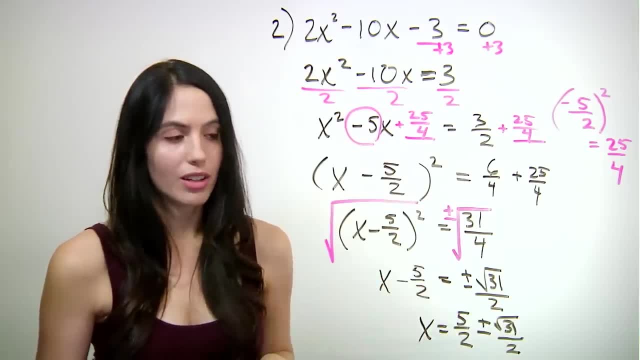 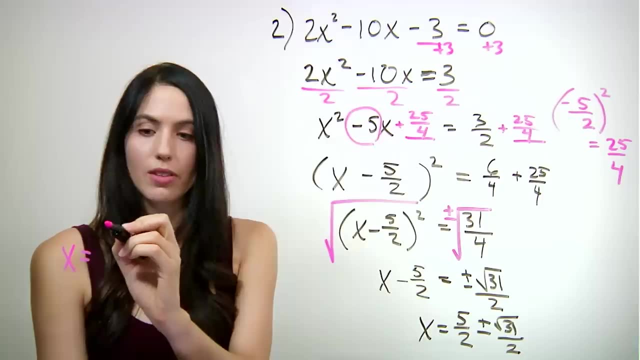 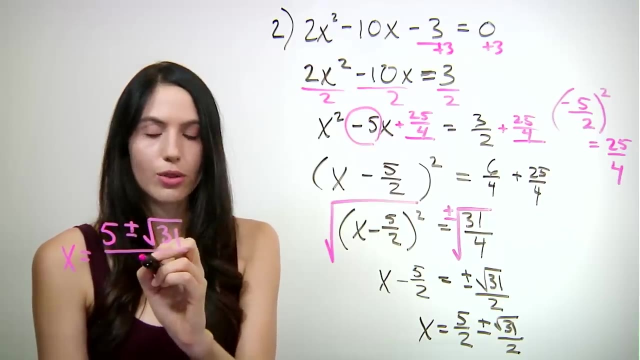 which most people would consider simpler. So you may want to do that, And your final answer would look like this: x equals 5.. Plus or minus square root, 31 as your numerator, all over 2 as your denominator. So these are your two solutions. 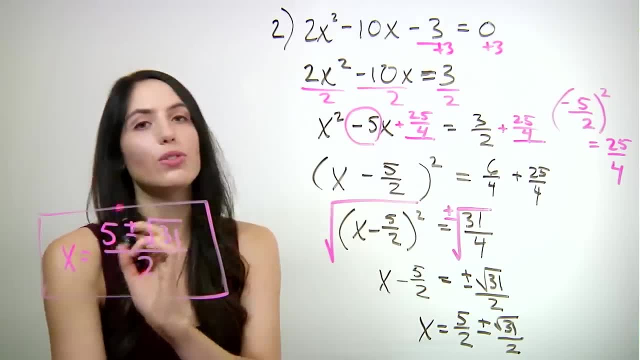 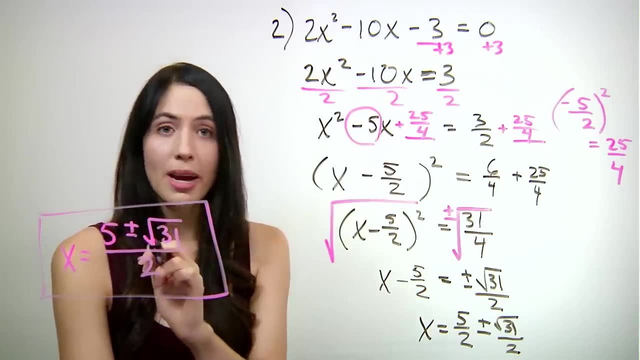 you got from completing the square. It may not look like it, but this is two solutions because you have two versions. You have 5 plus square root of 31 all over 2, and you have 5 minus square root of 31 all over 2.. 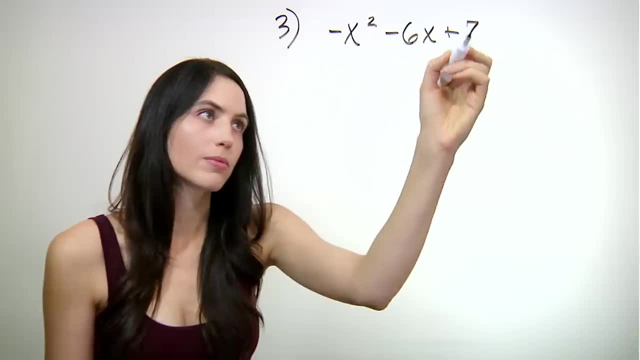 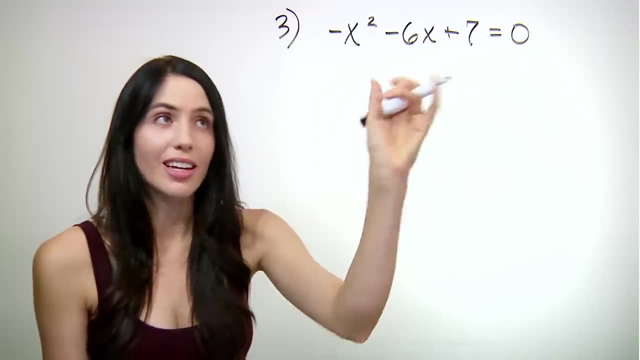 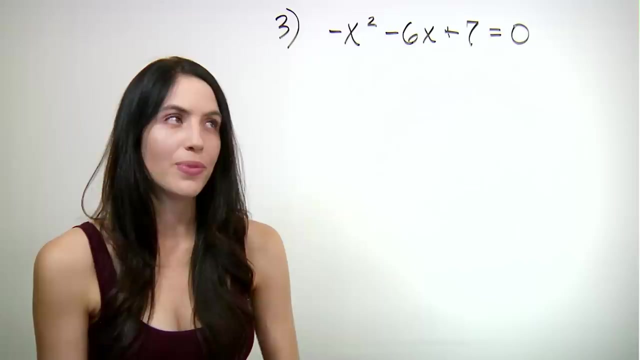 So those are your answers. Okay, say you have an equation that looks like this: It starts with a negative x squared, or negative 2x squared, where the coefficient of x squared is a negative number. Your first step will still always be. 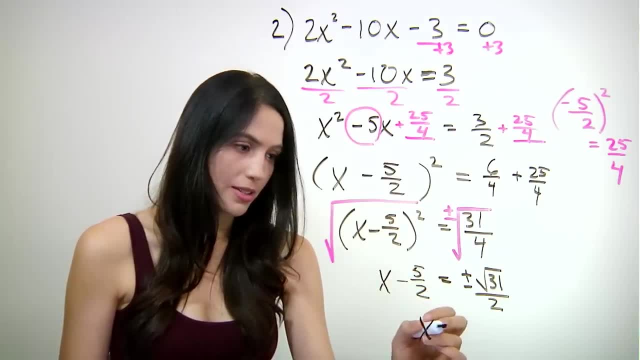 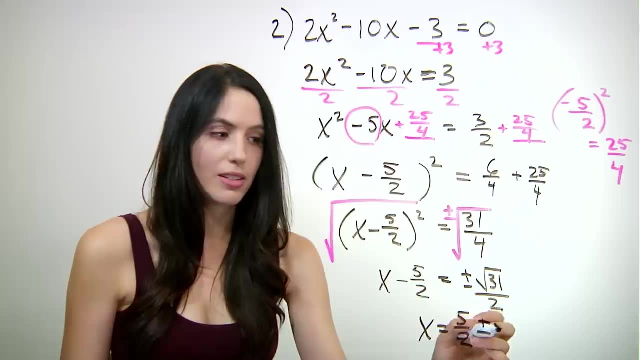 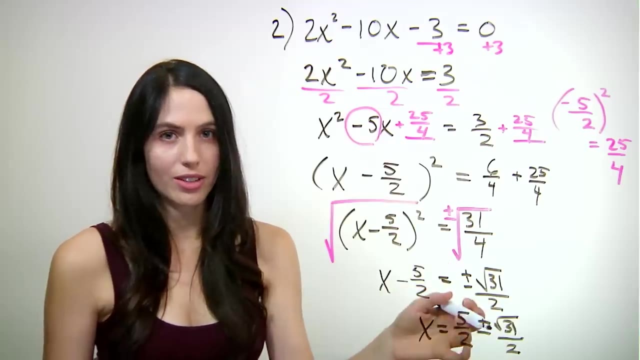 And your two solutions will be: x equals 5, halves plus or minus root 31 over 2.. You can actually combine this into one fraction. You can actually combine this into one fraction. You can actually combine this into one fraction, which most people would consider simpler. 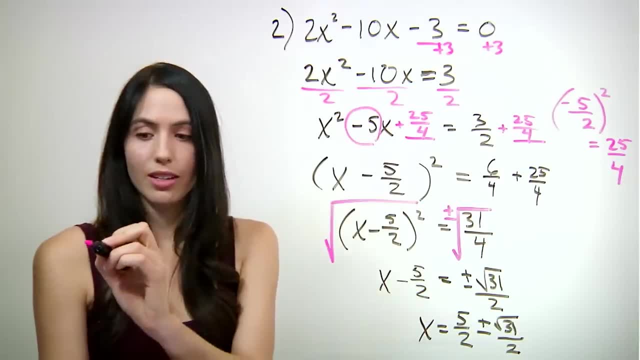 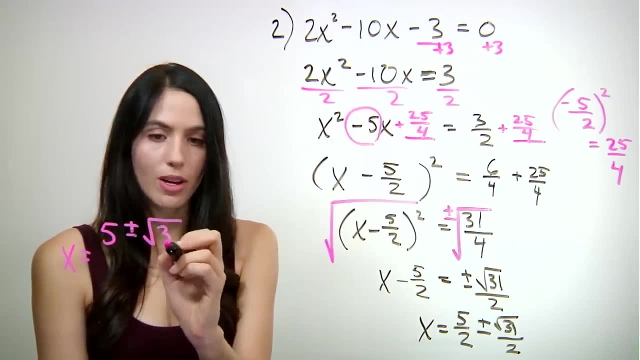 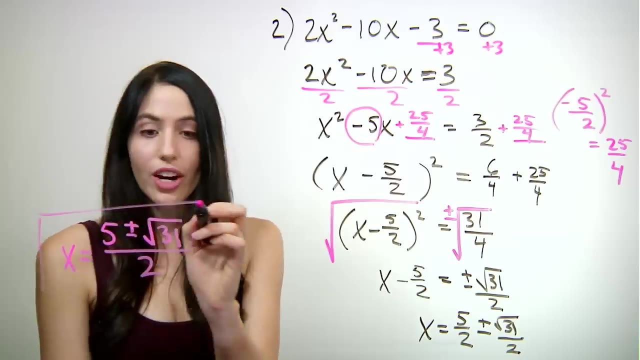 So you may want to do that, And your final answer would look like this: x equals 5 plus or minus square root, 31 as your numerator, all over 2 as your denominator. So these are your two solutions you got from completing the square. 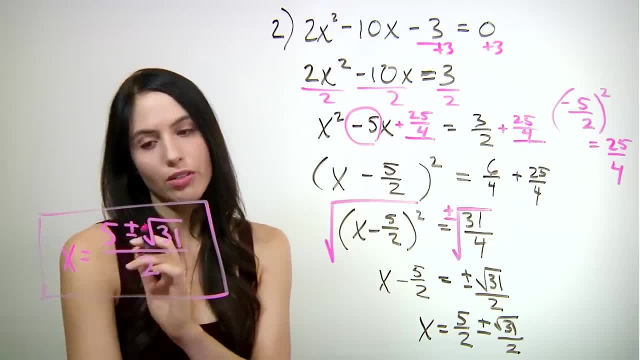 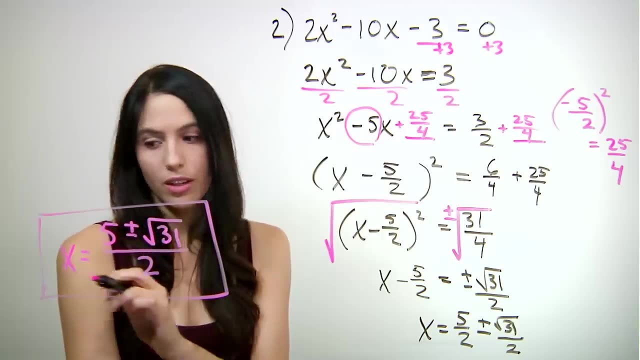 It may not look like it, but this is two solutions, because you have two variables: You have 5 plus square root of 31 all over 2, and you have 5 minus square root of 31 all over 2.. So these are your answers. 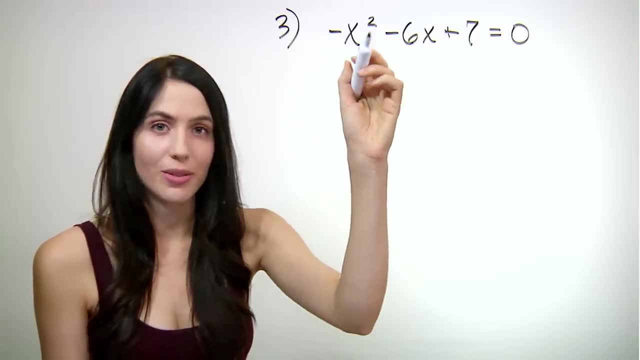 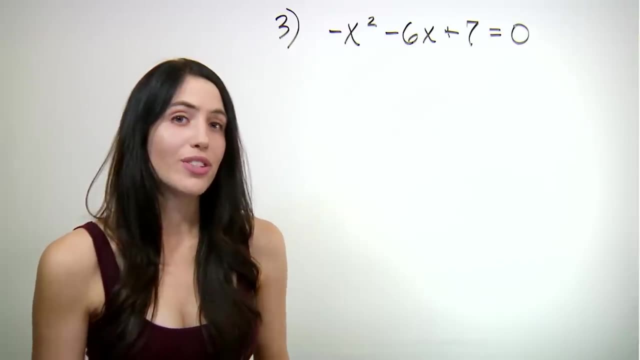 Okay, Say you have an equation that looks like this that starts with negative x squared, or negative 2x squared, where the coefficient of x squared is a negative number, Your first step will still always be to move the constant over to the right hand side. 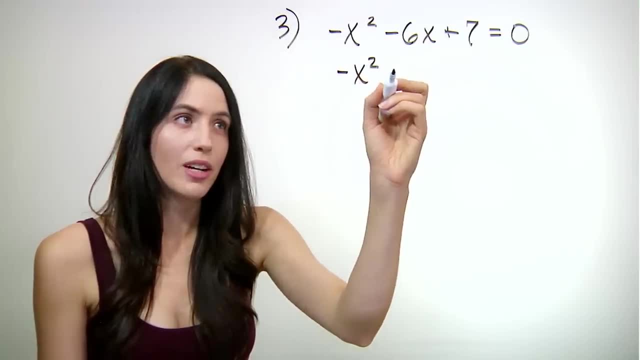 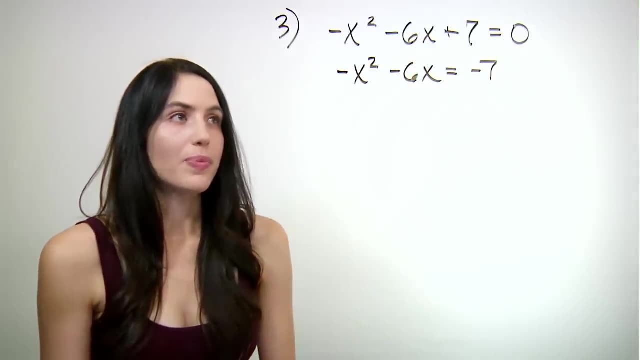 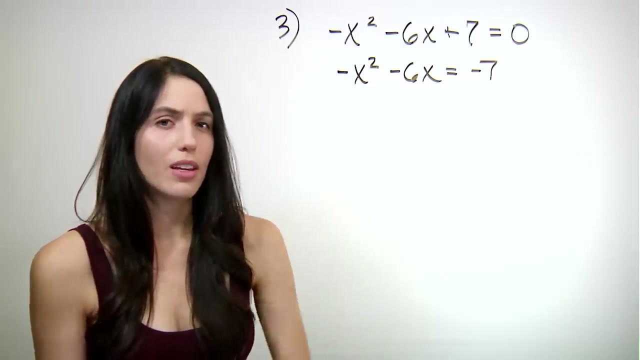 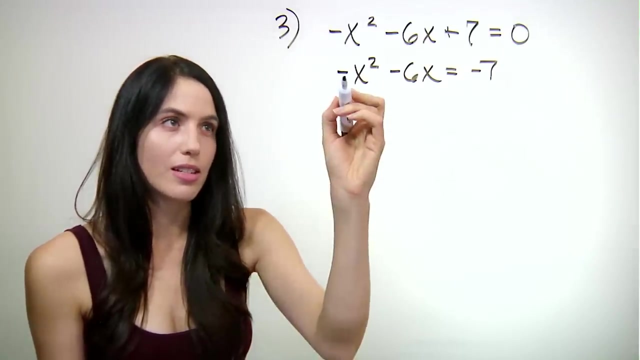 So the next line: you would have negative x squared minus six. x equals negative seven. Notice the sign changed. And then you don't want the negative in front of the x squared before you complete the square, So you actually will divide every term by a negative one to get rid of it. 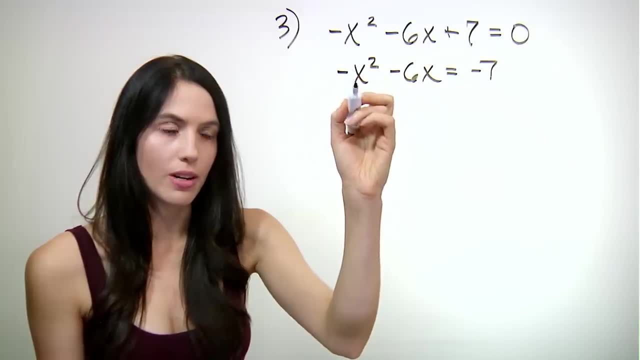 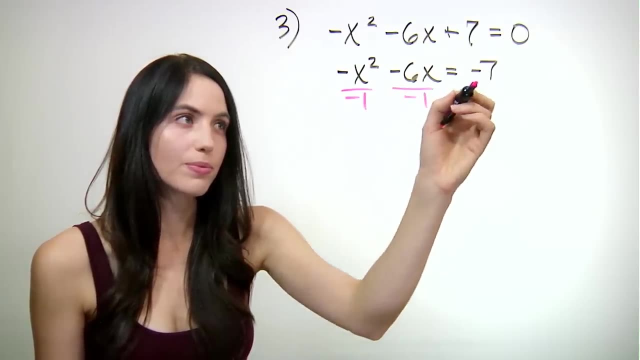 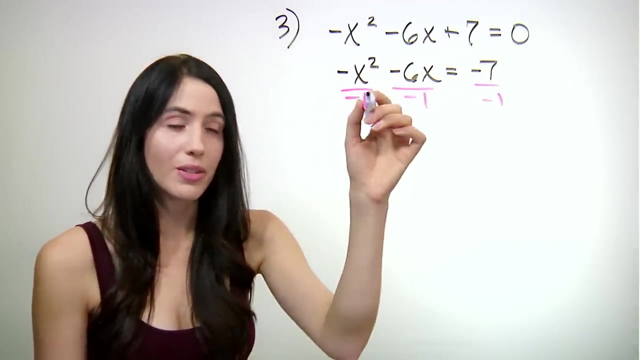 Since there actually is a negative one here. you don't see the one, but you can divide every term by negative one, even the right hand side, And what that does is it flips the sign of every term. So, instead of negative, x squared. 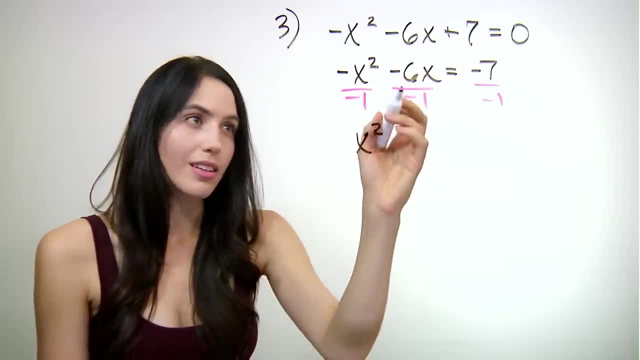 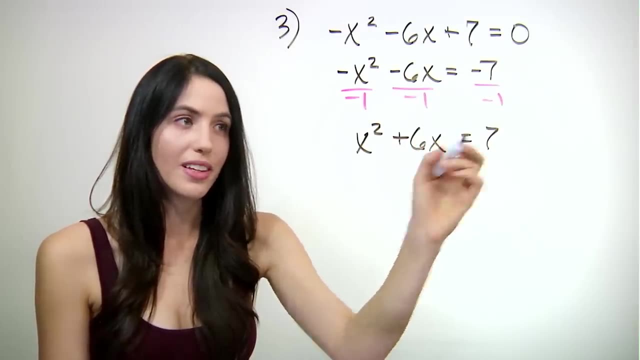 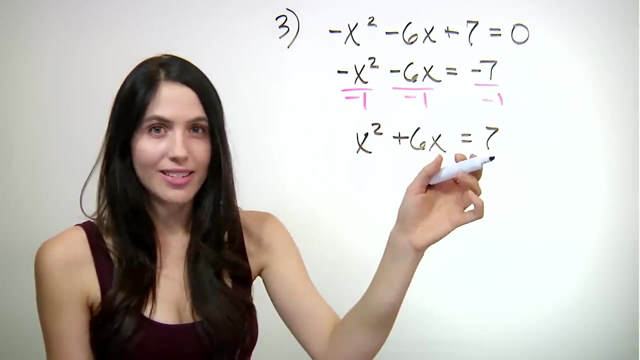 you'll have positive x squared, which you want, positive six x and on the right side, positive seven, And then your steps from there will be the same as in problem one and two, Adding a number to both sides that you get. 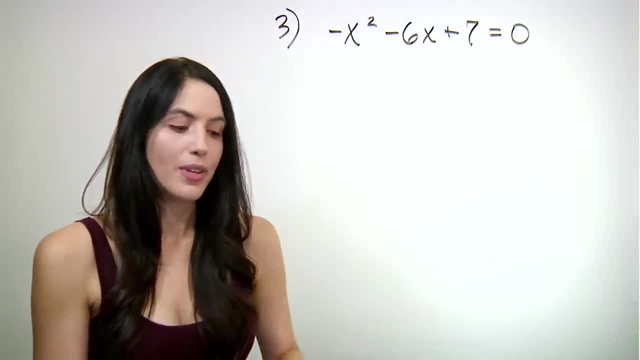 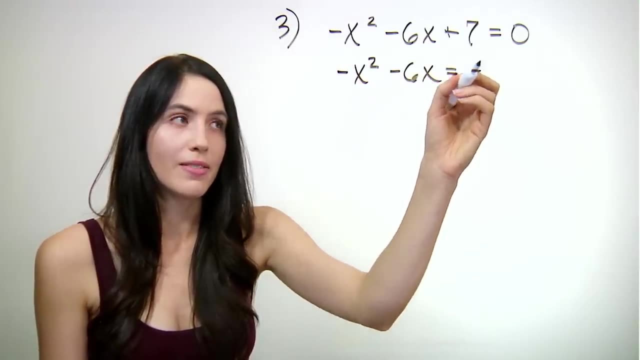 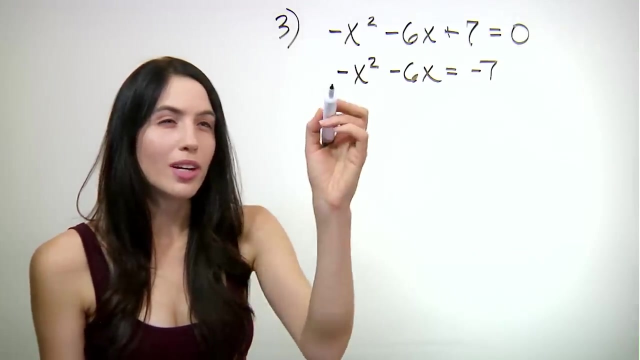 to move the constant over to the right-hand side. So the next line you would have negative x squared minus 6x equals negative 7. Notice the sign changed. And then you don't want the negative in front of the x squared before you complete the square. 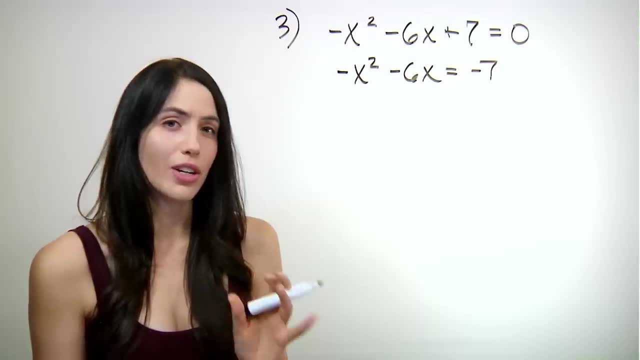 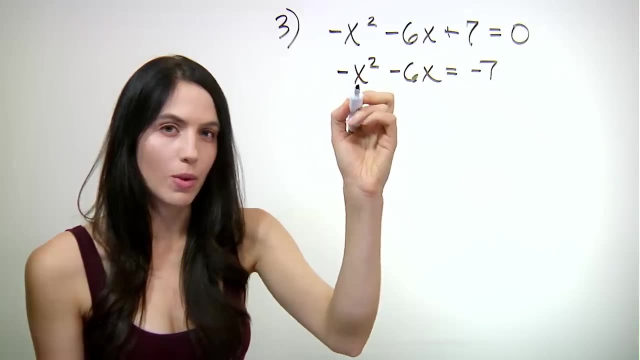 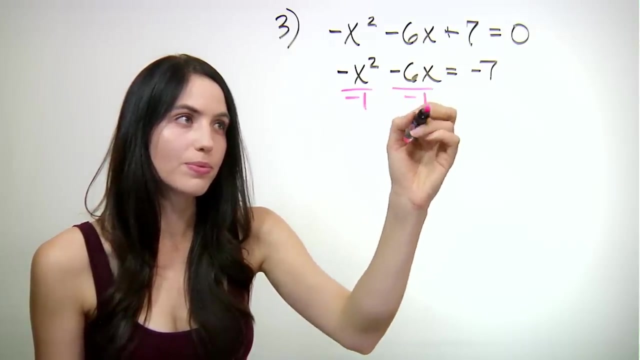 So you actually will divide every term by a negative 1 to get rid of it. Since there actually is a negative 1 here, you don't see the 1, but you can divide every term by negative 1, even the right-hand side. 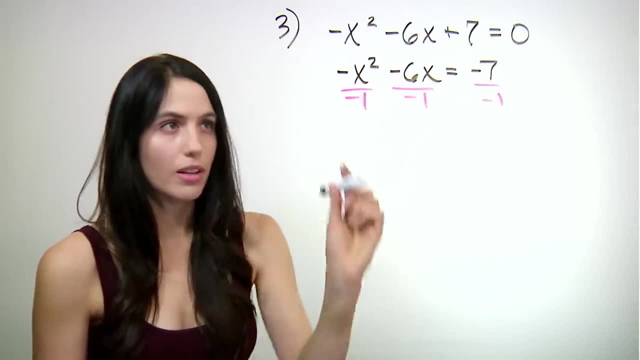 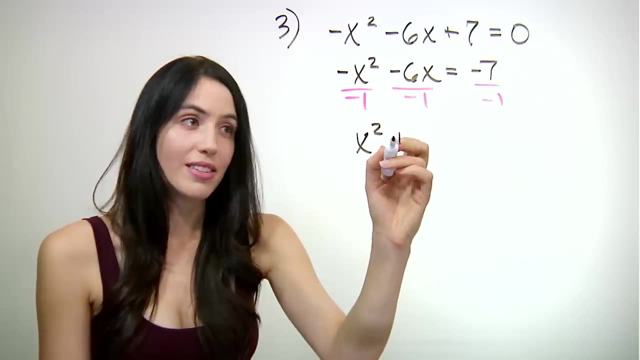 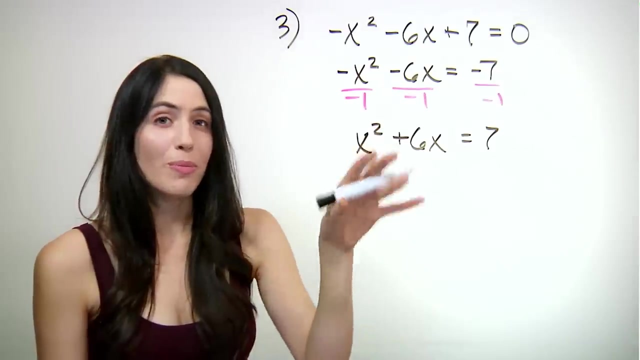 And what that does is it flips the sign of every term. So, instead of negative x squared, you'll have positive x squared, which you want, positive 6x and, on the right side, positive 7.. And then your steps from there. 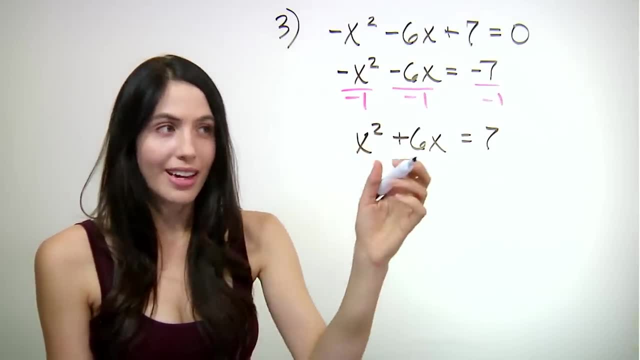 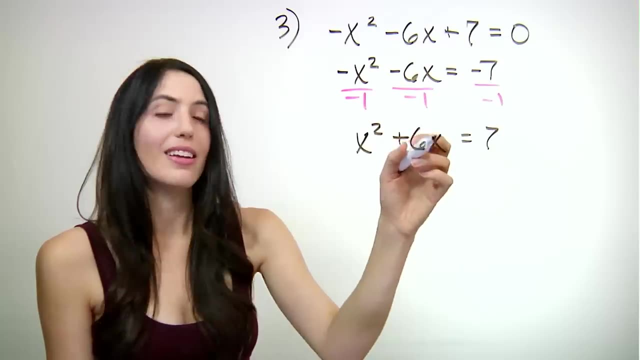 will be the same as in problem 1 and 2, adding a number to both sides that you get from dividing this number by 2 and squaring it. So you would add 9 to both sides: 6 over 2 squared 9 to both sides. 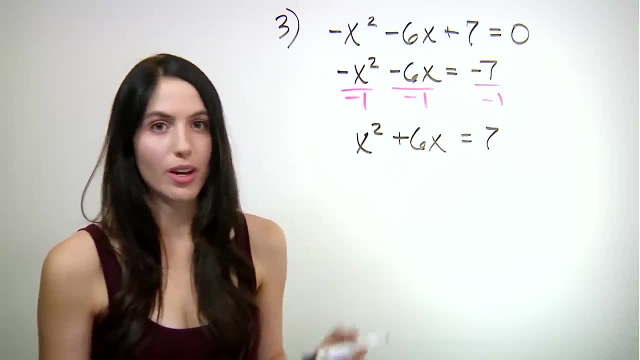 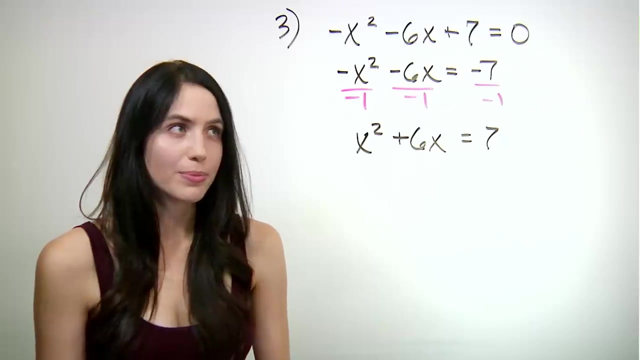 Writing it as a perfect square solving by square rooting both sides. From then on it would be the same. So notice this is a lot like case number 2, example number 2, where you divide out anything that was in front of x squared. 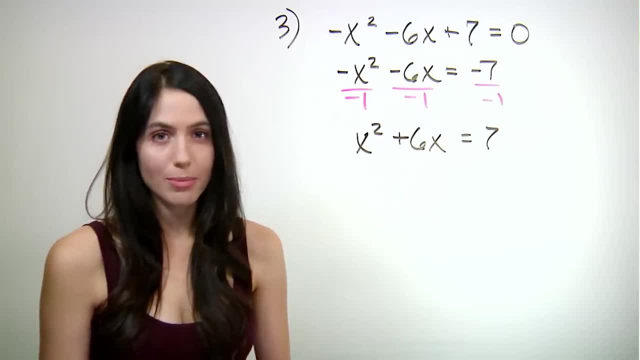 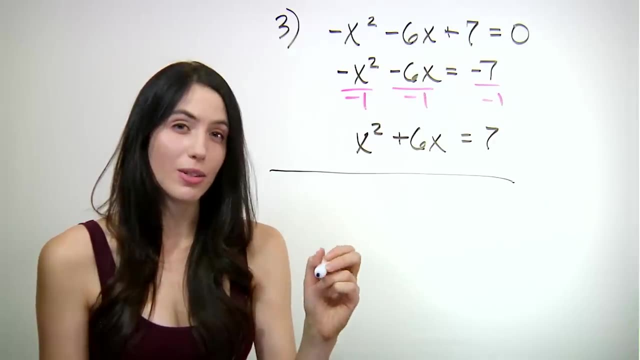 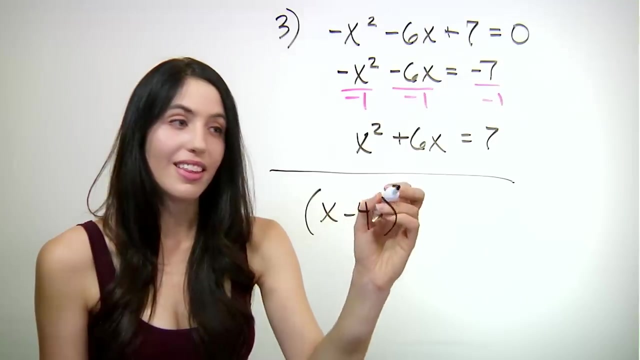 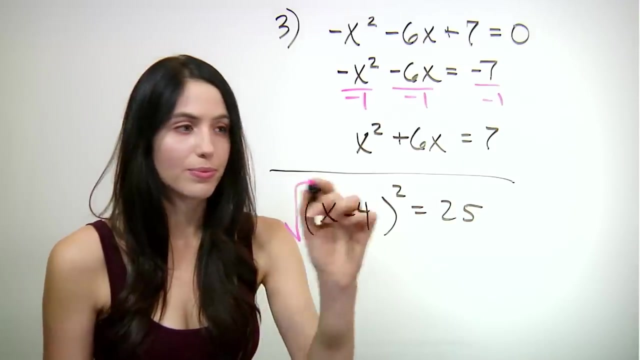 Okay, things that tend to trip people up about completing a square. The biggest thing is forgetting to put plus and minus in the solution. So if you get to the point where you have an equation that looks like this, when you square, root both sides to solve, 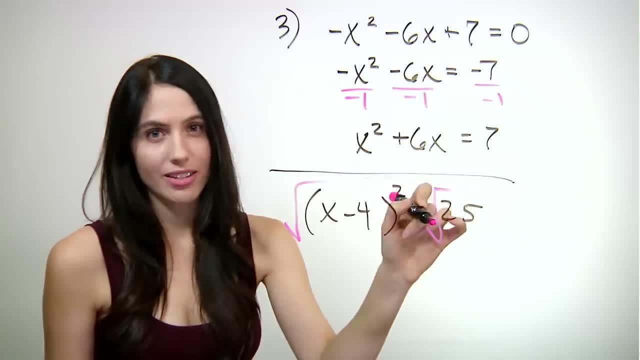 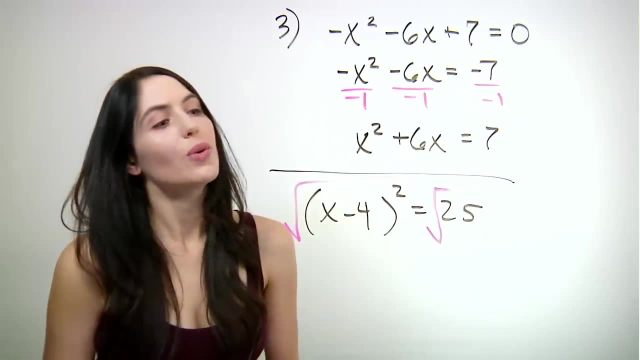 a lot of people forget to put plus and minus here on the constant side and just write the root. Lots of people forget that You don't want to miss the other solution. There are two solutions. And if you don't put the plus and minus, 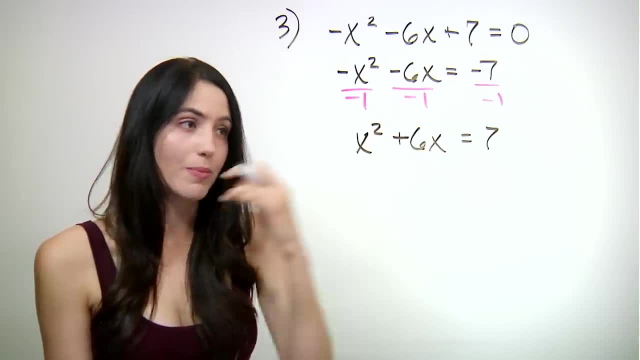 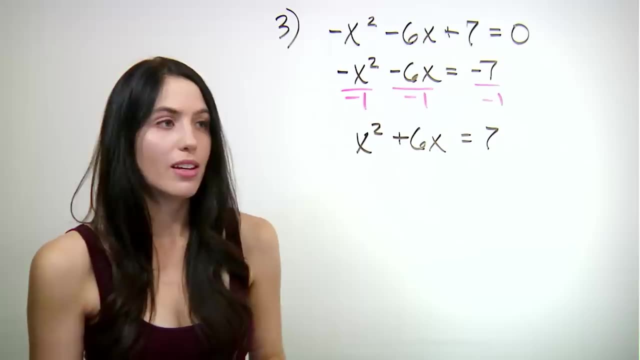 from dividing this number by two and squaring it, So you would add nine to both sides, Six over two, squared nine to both sides, Writing it as a perfect square solving by square rooting both sides. From then on, it would be the same. 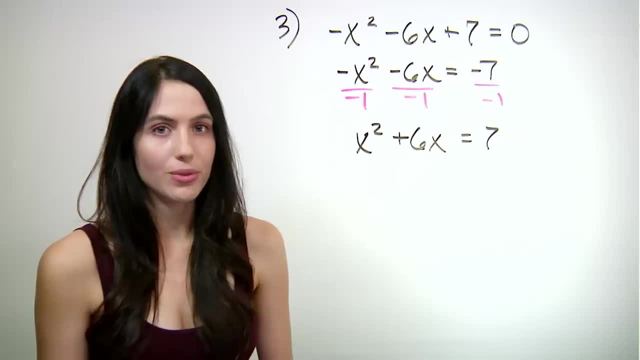 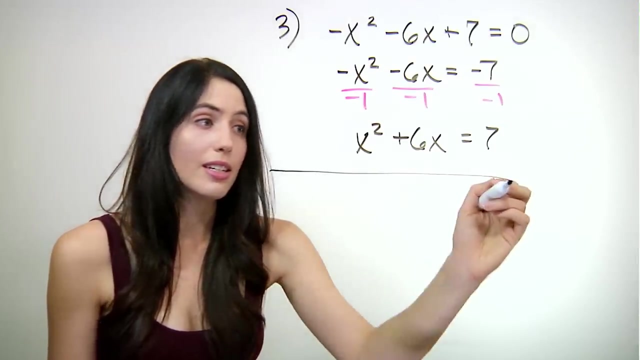 So notice this is a lot like case number two, example number two, Where you divide out anything that was in front of x squared. Okay, things that tend to trip people up about completing a square. The biggest thing is forgetting to put plus and minus. 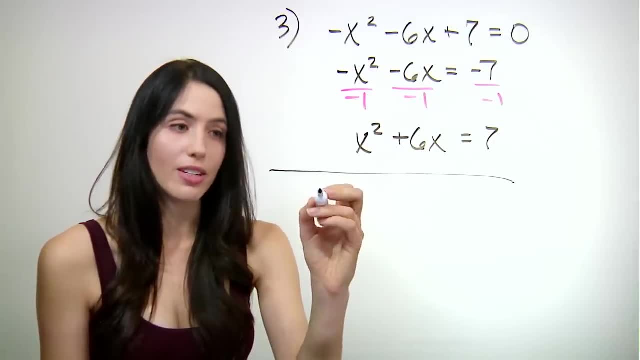 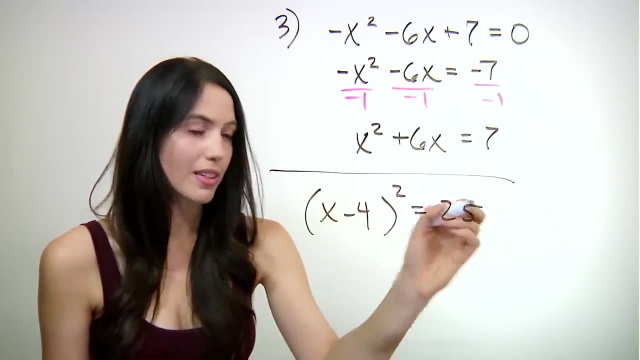 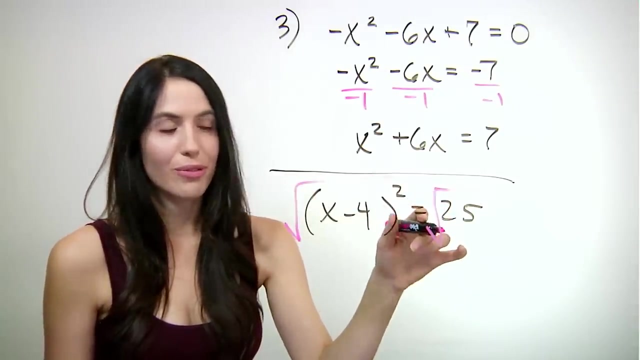 in the solution. So if you get to the point where you have an equation that looks like this, When you square root both sides to solve, a lot of people forget to put plus and minus here on the constant side And just write the root. 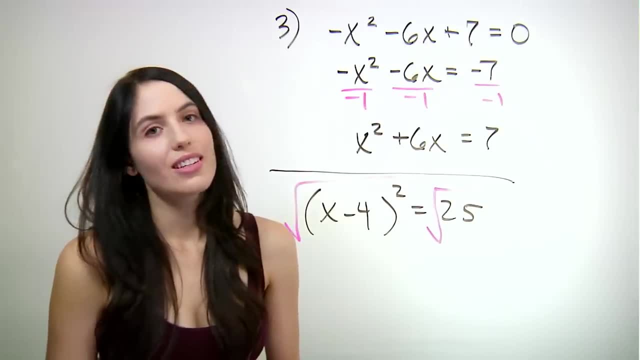 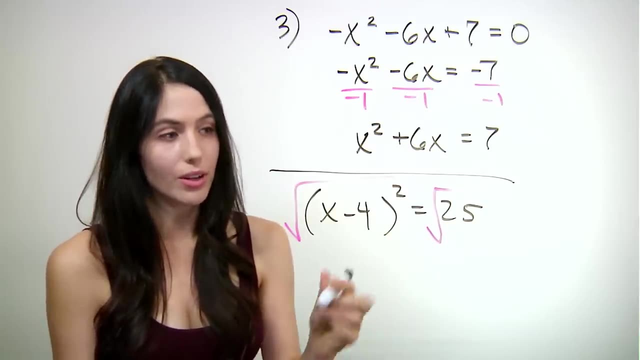 Lots of people forget that. You don't want to miss the other solution. There are two solutions And if you don't put the plus and minus, you're only getting the positive solution. So remember the plus and minus. a lot of people forget that. 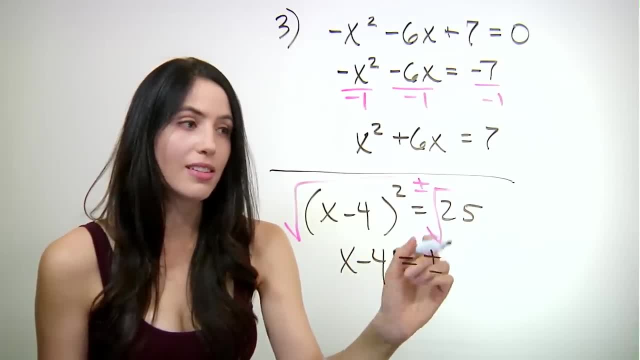 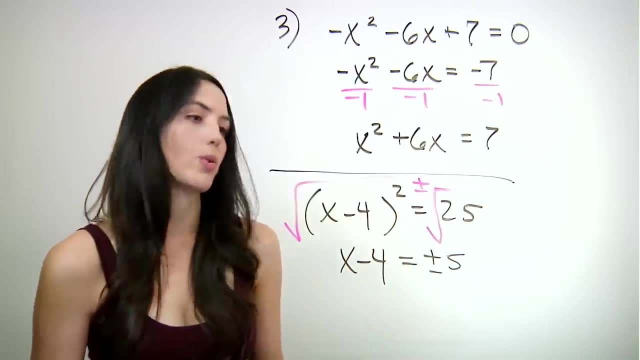 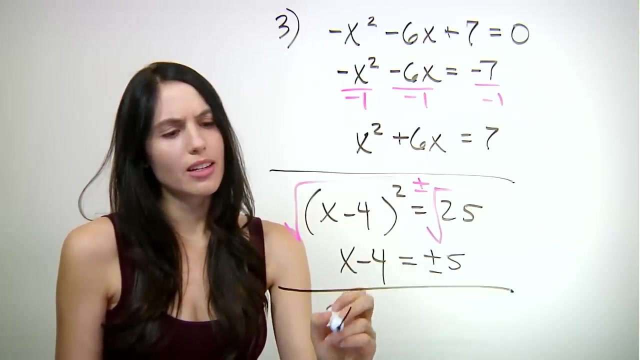 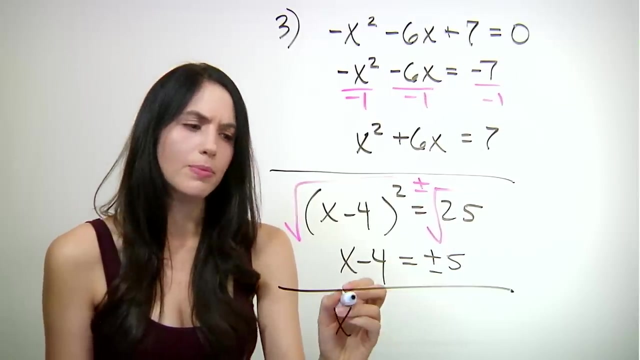 You just have x minus four equals plus and minus Plus five in this case, And you would keep solving from there. So that's the biggest thing people forget when completing the square. Another thing that trips people up is sometimes they think you can complete the square if there's no x term. 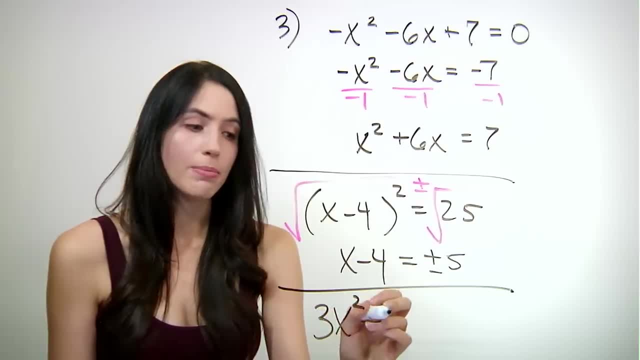 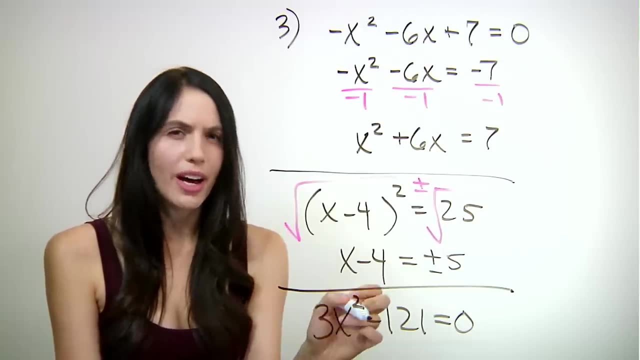 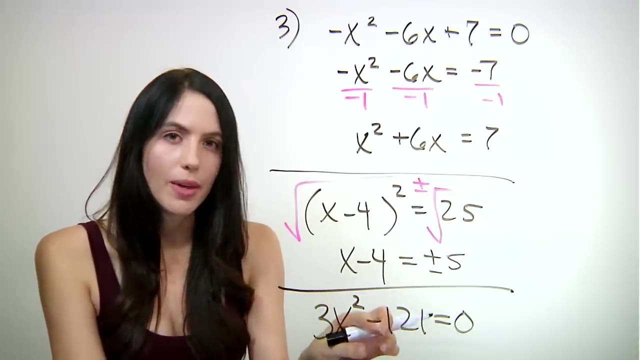 For instance, if you had three x squared minus 121 equals zero. if that was your equation, You can't complete the square because you have no x term, Such as three x squared plus 10x minus 121.. If there's no x term there, you have no coefficient. 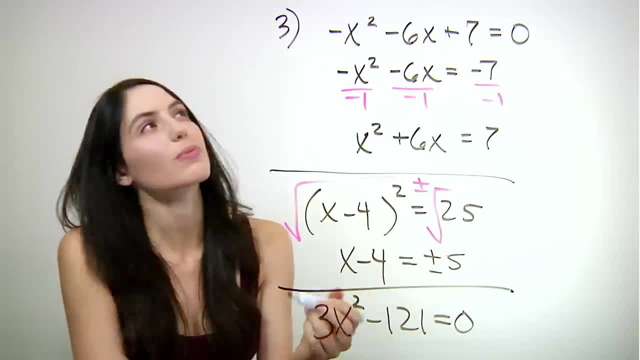 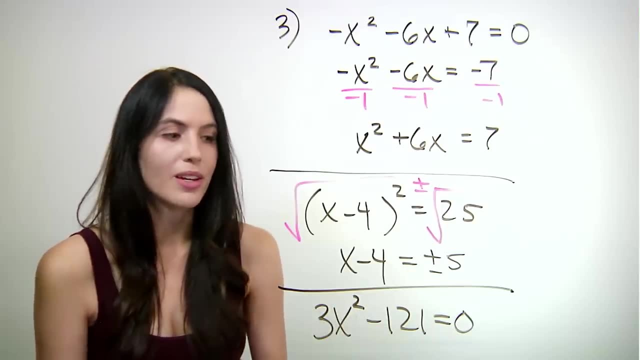 to use when adding a number both sides. So you can't complete the square. if it looks like that, You'll have to use another method, So factoring quadratic formula, something like that. So I hope that helped you understand how to solve. 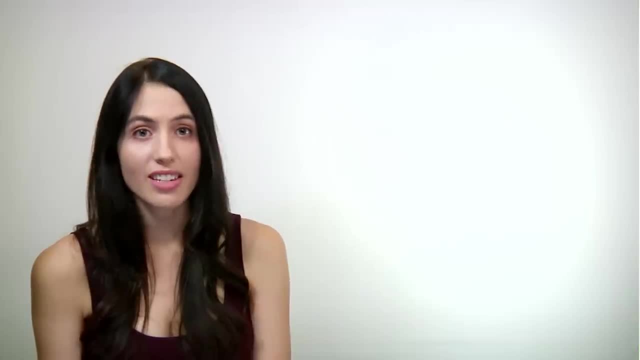 by completing the square. Completing the square is fascinating. No, It's okay, You don't have to like it, but you can like my video, So if this helped you, please click like below.